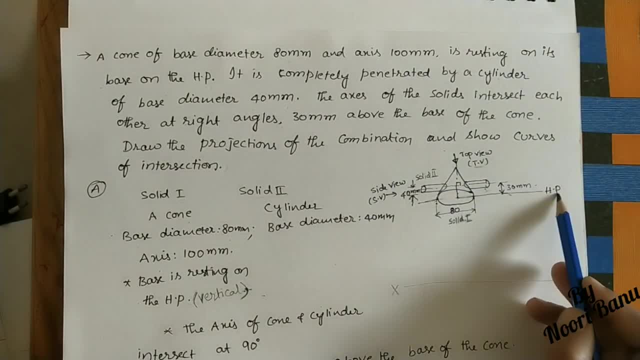 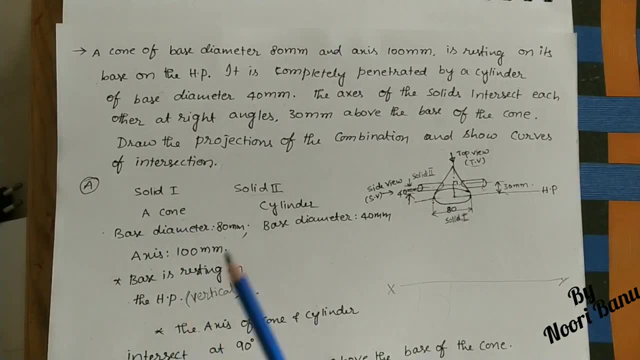 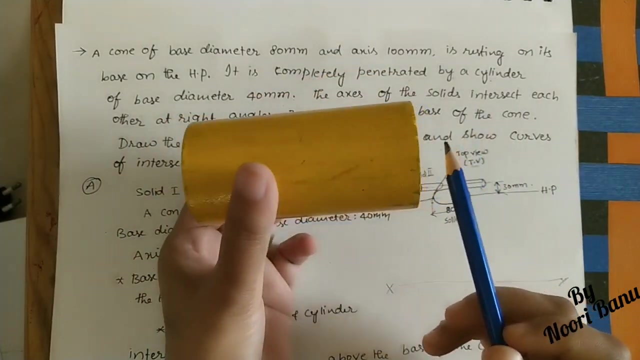 position, just roughly i did solid one position like this: this base is on the horizontal plane and this diameter is 80 mm and height is 100 mm. okay, these are the given conditions for the solid one cylinder means it is the solid two. okay, it has. this is the cylinder. it has two faces. 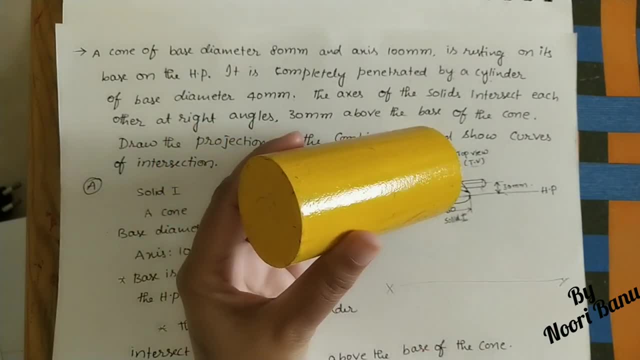 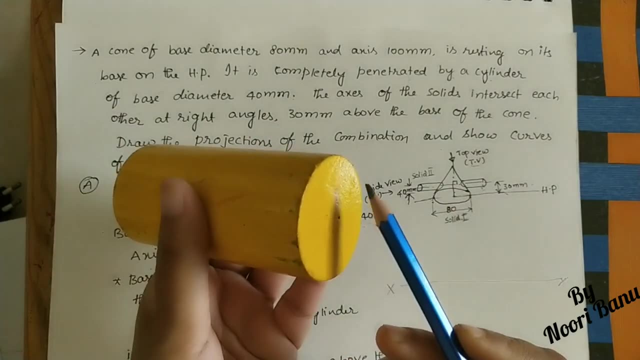 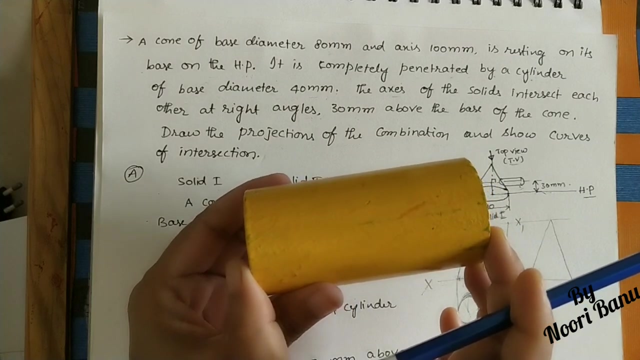 these are circular one. these two faces are in the form of circles. okay, so the solid two is a cylinder. and then it has base diameter: 40 mm. same thing i have written here. this is one of the face or base we can call. it is 40 mm and this is also 40 mm height. has not given this length or height has. 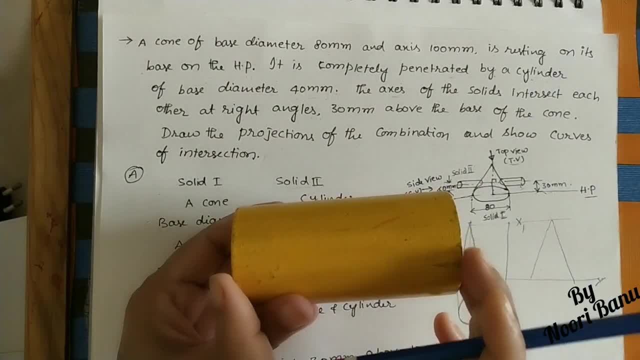 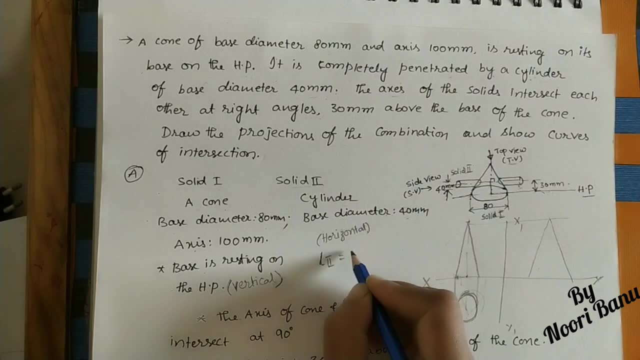 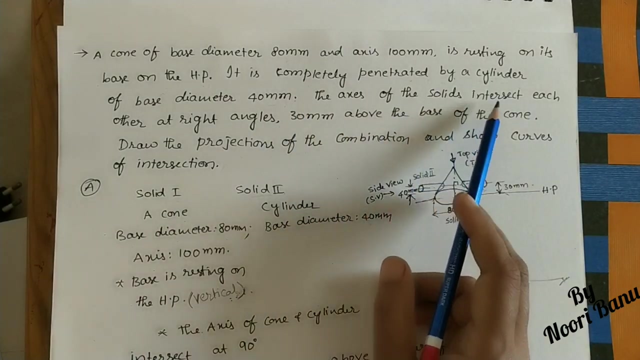 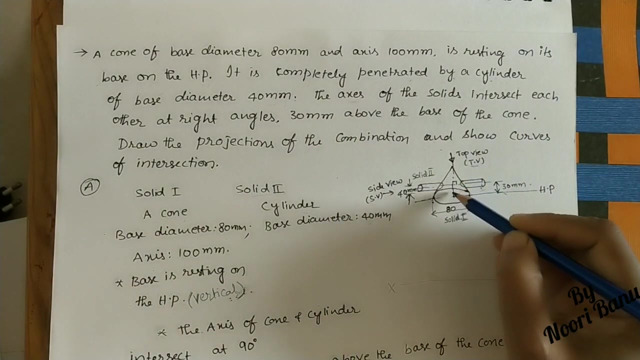 not given. whenever values are not given. take 100 mm. okay, height or length. so i am taking this height and this length is length of the solid. two: okay, it is 100 mm. do push-up. the axis of the solids intersect each other at right angles. okay, if you are taking access here, axis means it is a imaginary line. okay, two big lines with one dot. 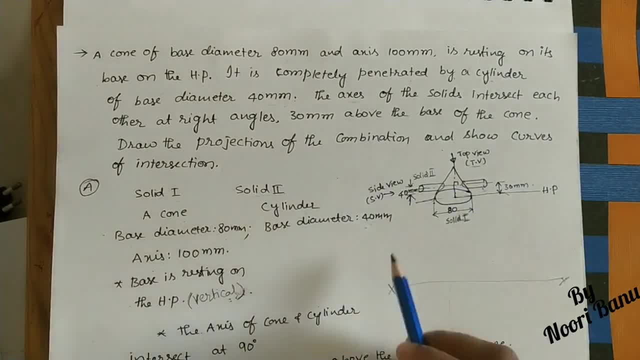 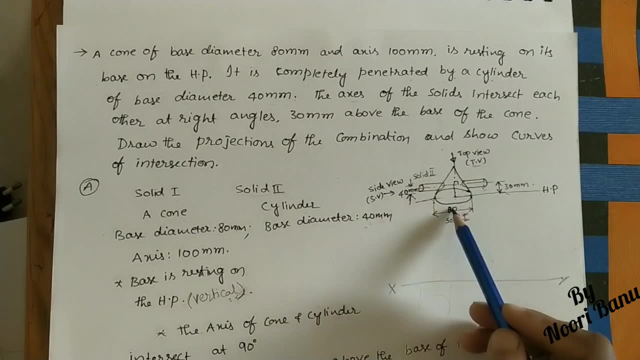 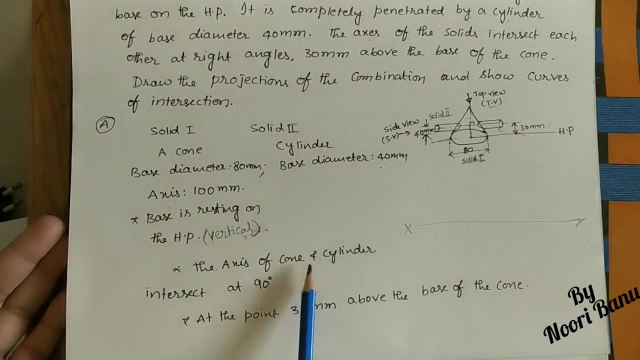 okay, access. this is the axis of the cone. okay, and here i did the cylinder like this: and this imaginary line is the middle line, is the axis line. these two axes are intersect at each other at 90 degrees. okay, so, same given thing i have written here: the axis of the cone and cylinder intersect at 90 degrees, or we can call it as right angle. 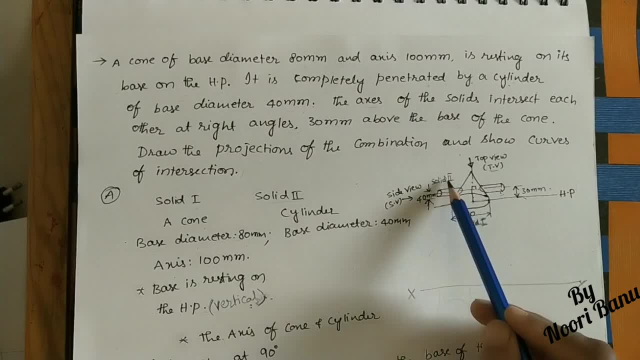 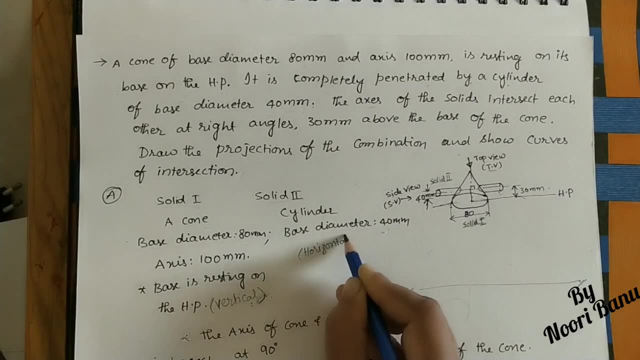 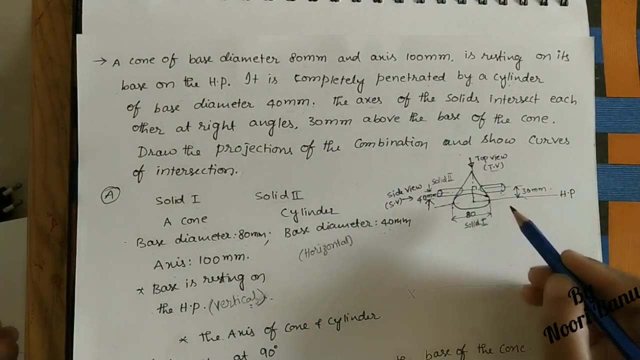 to each other. okay, so the position of the second solid, that is, cylinder, is horizontal. okay, just i will write here horizontal so roughly i did that 3d diagram here and next, given data is: and 30 mm above the base of the cone, the intersection point is: this point is okay, it is the intersection point of this cylinder. 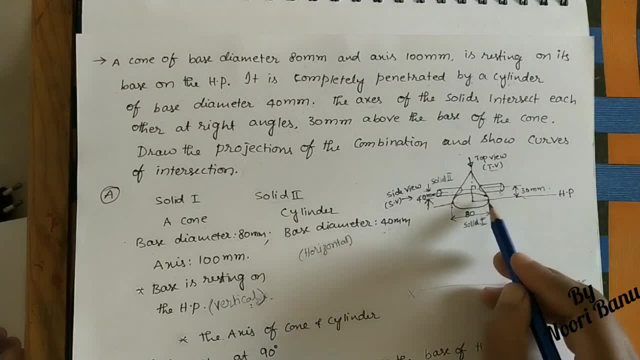 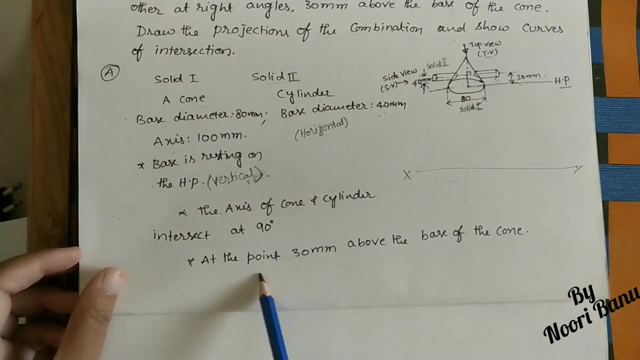 and this cone. okay, this point is 30 mm above the hp, above the ground. okay, just now i told this this base is on hp. okay, here i have written from the ground it is 30 mm. this point is okay. so i have marked 30 mm here. okay, same thing. i have written here: 30 mm above the. 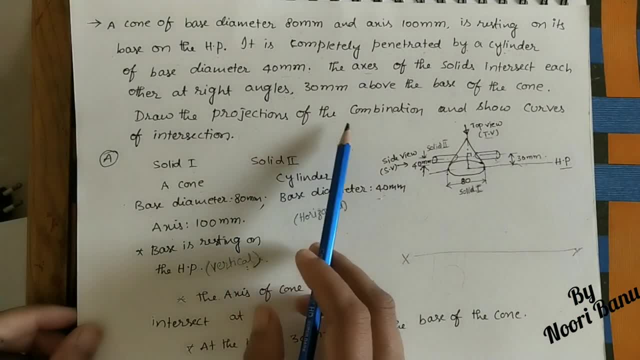 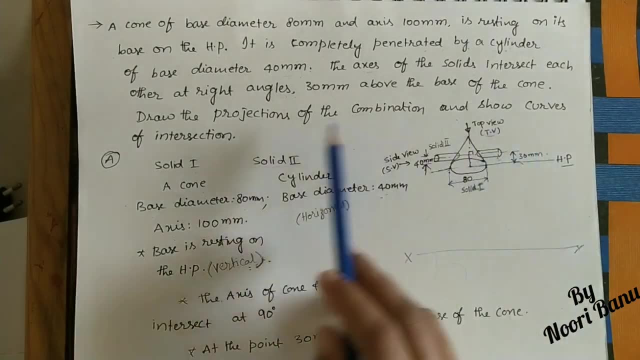 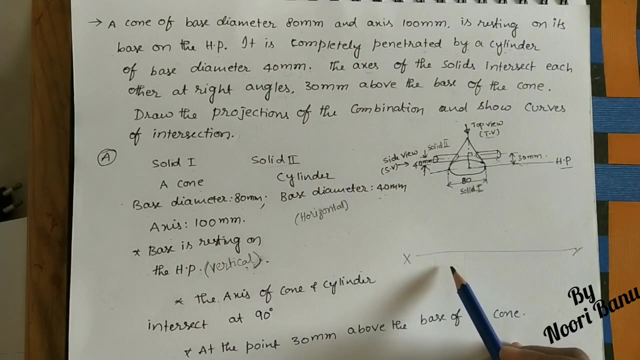 base of the cone, draw the projections of the combination. projections means so the projection is just now. i told front view, top view and side. with three views we have to draw and show curves of intersection. after getting the projections we can draw the curves of intersection. okay, initially we will do the rough diagram here for the 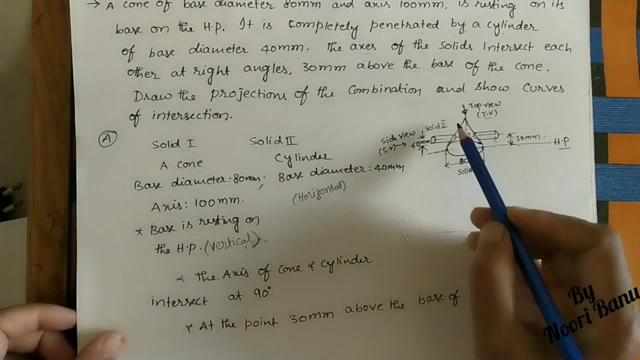 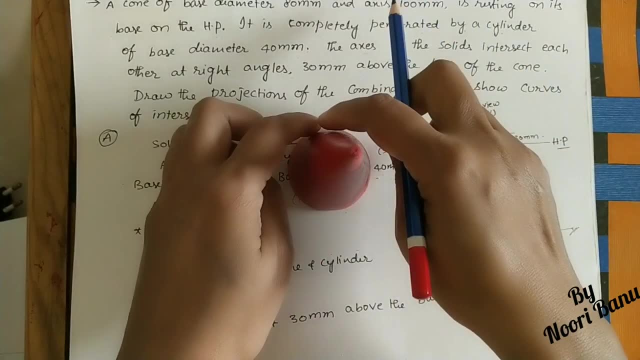 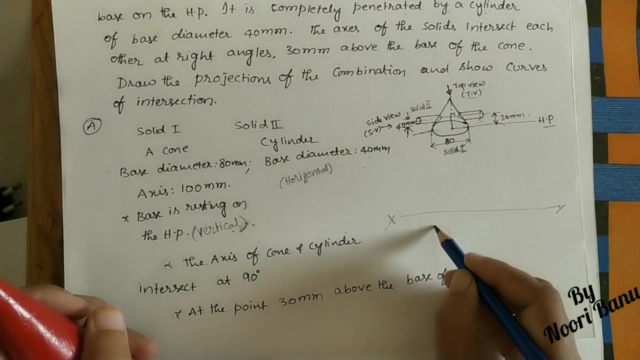 solid one projections, which is a solid one cone. okay, this is the cone. okay, first, initially, we will do the top view. okay, if you see from top for the cone, okay, we can see the circle which is on the horizontal plane. so, for doing it, just do one xy line of any length we can. 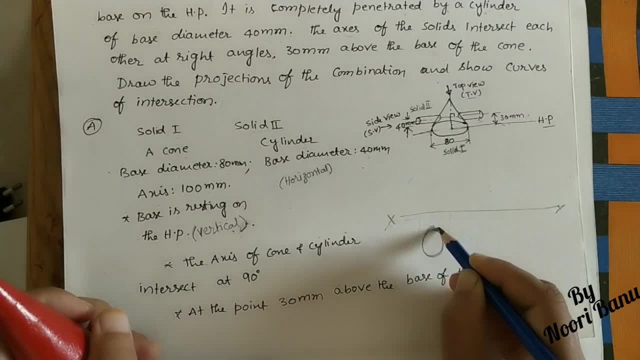 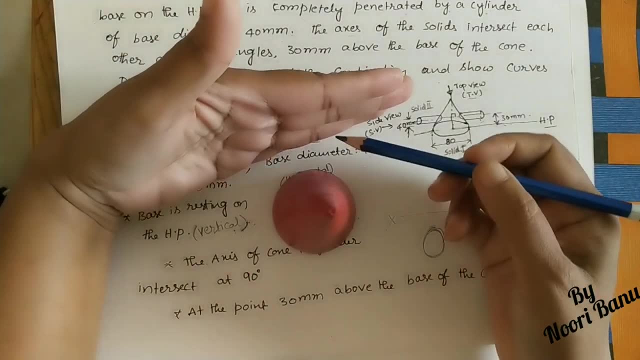 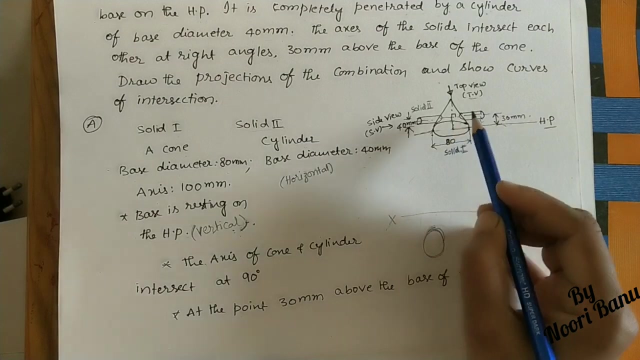 do one xy line right and then another xy line, okay, so this is the circle here. okay, roughly, i am doing here without instrument. okay, this is the base of the cone. okay, now here, this gap is not given. let us take. this is a vertical plane. this gap has not given. okay, we can take. 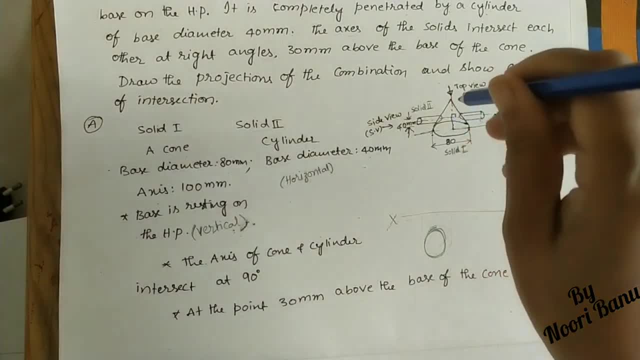 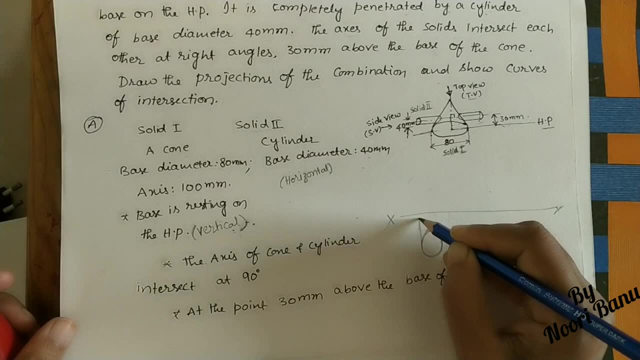 any gap from xy line. now, after doing the top view, do the front view. front view means we have to see from the front of this diagram like this: in the front view the cone is looking like triangle. the front view is coming above xy. just do the projector lines here as you. 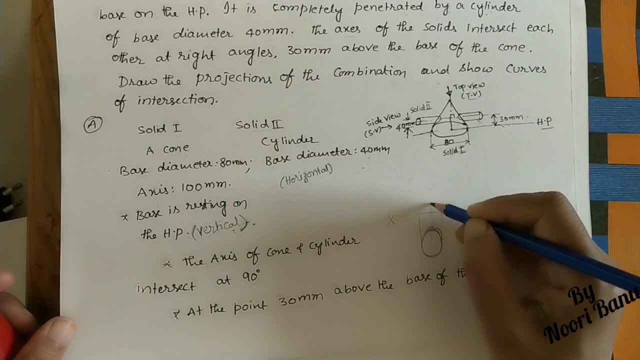 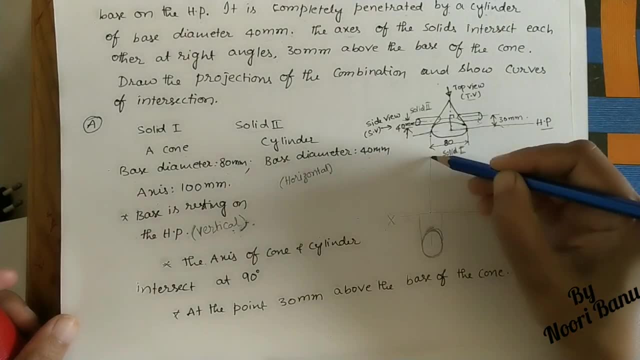 Projectile lengths means light color lengths. Do the axis? What is the height of the cone? They have given 100 mm. So from here, take 10 cm from this point to this apex. This is called apex. Okay, Now we can see the triangle here. 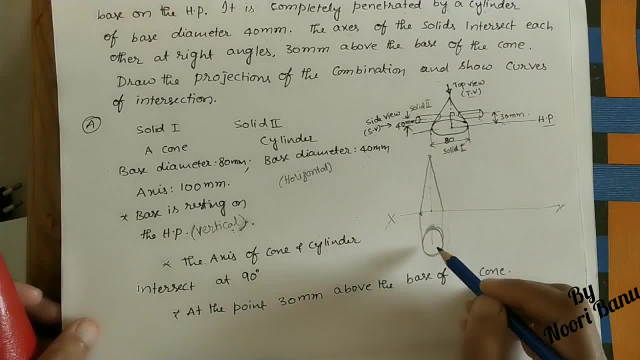 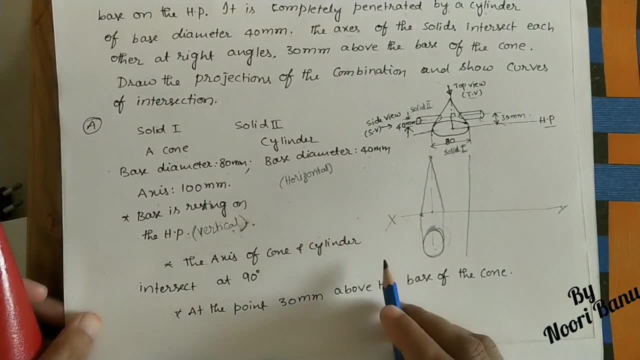 Like this: Now, this is the top view, This is the front view. We will do the side view here. For doing the side view, first do the reference line. One more reference line similar to like this: Here, instead of same xy, I am giving x1, y1.. 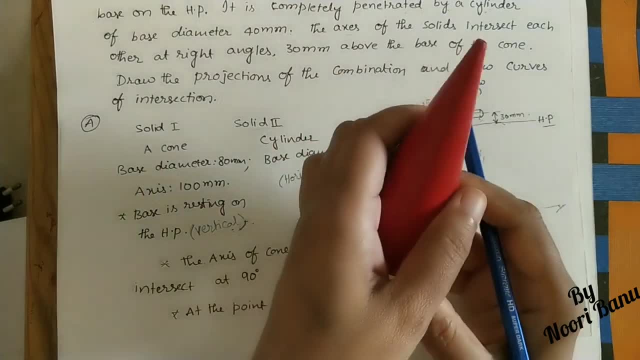 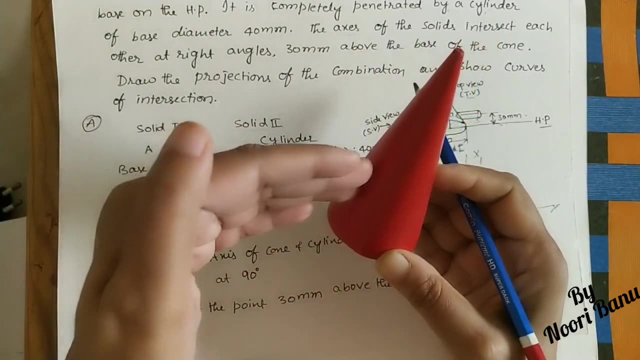 Do the side view of the cone only. If you see, this is the front view We did here And side view also looking like similar to the front view. Okay, So it is also looking like triangle here. Here we will get side view. 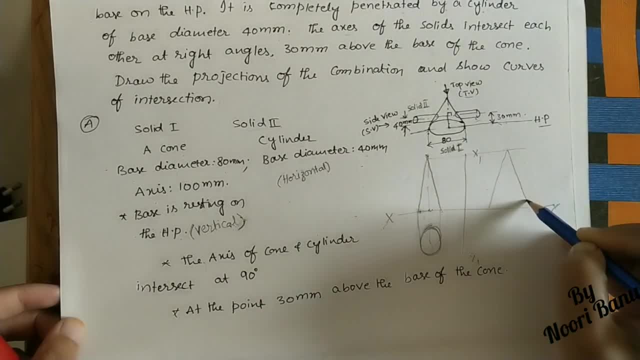 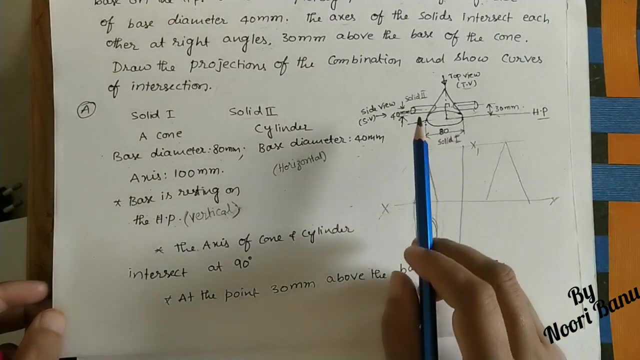 Okay, Roughly, I am doing of the same height Like this. First, initially we will do the front view, top view and side view of the solid one By using the drawing instrument. After that we will do the solid to projection. This is also in it. 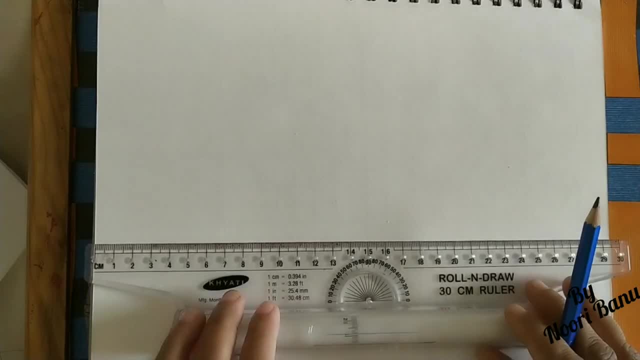 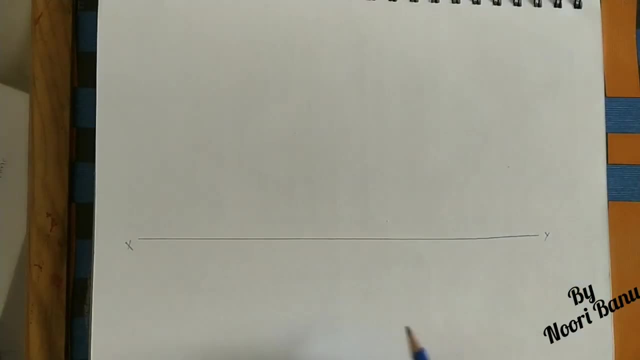 Let us do the xy line of some length by using scale. After getting this line xy, line mark xy. Here do the top view of solid one. Okay, Solid one top view is circle. What is the diameter of the circle? 80 mm. 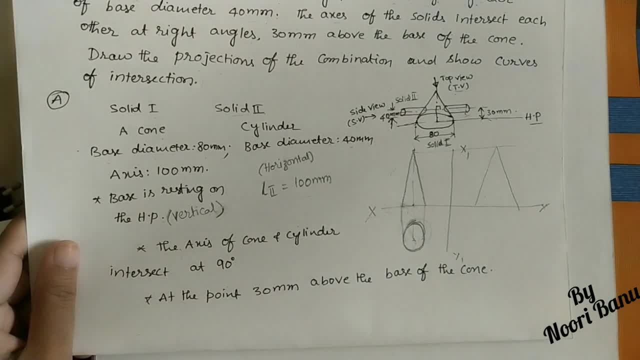 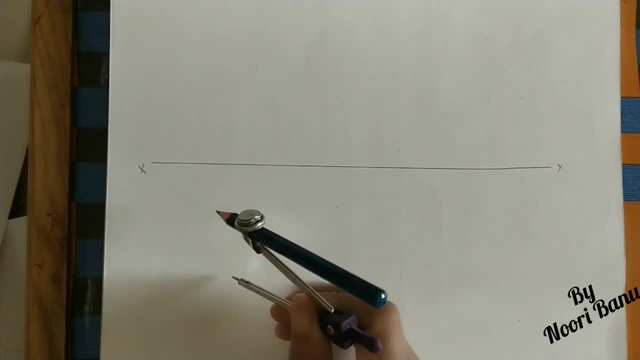 Okay, This is 80. Radius is 40 mm. That is 4 cm By using compass. take 4 cm Here. take 4 cm radius Below, xy. Take any one of the point as center, Just do one circle. 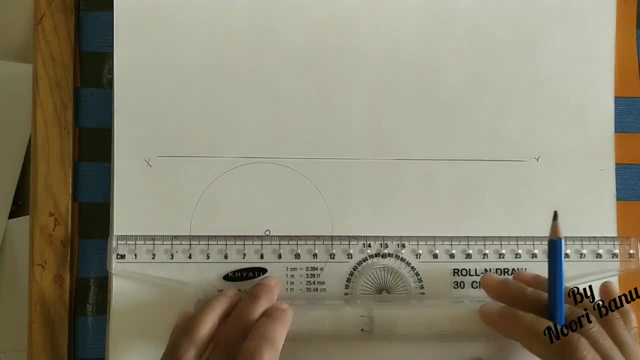 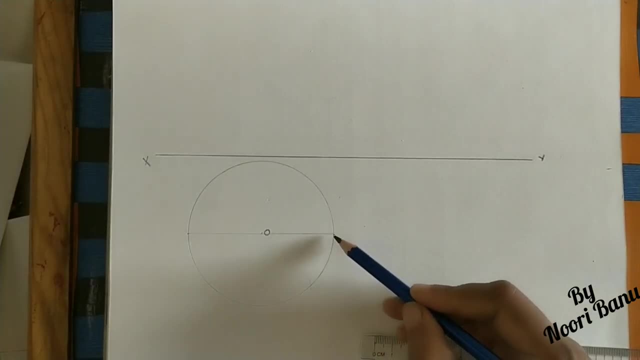 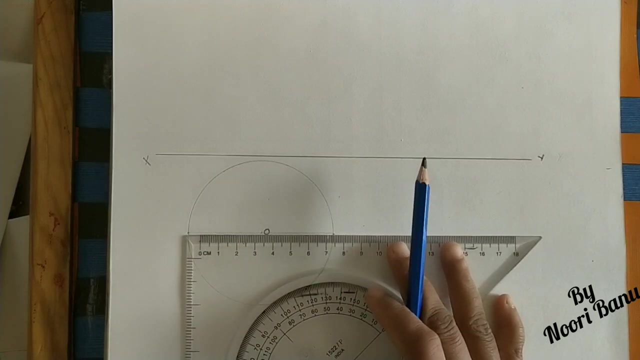 So take, this is the reference line. Move the scale Here, do the horizontal diameter. After getting these points, do the projectile lines at these points. Projectile lines means 90 degrees to this xy line. Okay, So we draw after it is easy to do the parallel lines as well as vertical lines. 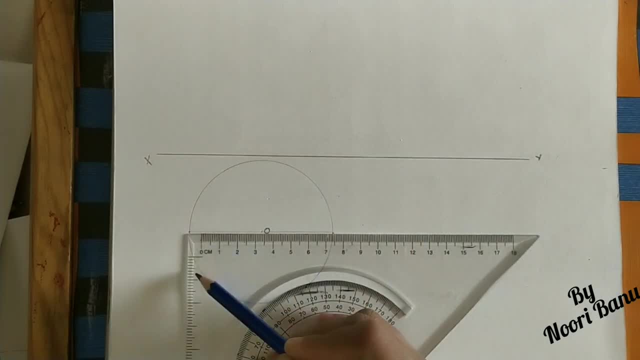 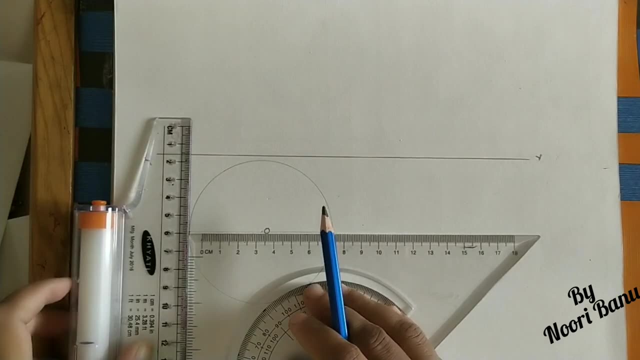 90 degrees. lines Here for getting 90 degrees. Okay, This is 90.. Okay, Here I will do one line by using scale. Perfectly, we will get the 90. So take this scale should coincide with this diameter. and here do the line. 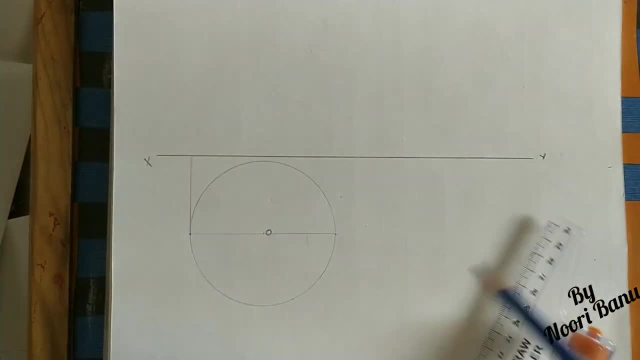 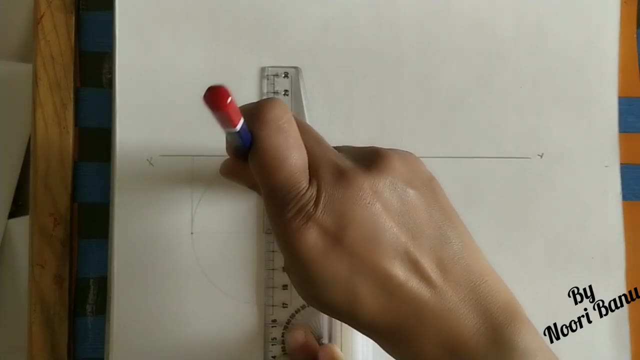 Take- this is the reference line for doing the line here- and I do the axis also here. Move the scale in this direction. Do the axis line here. Axis line means two big lines with a dot. Do up to some distance Here also do the kujakka line. 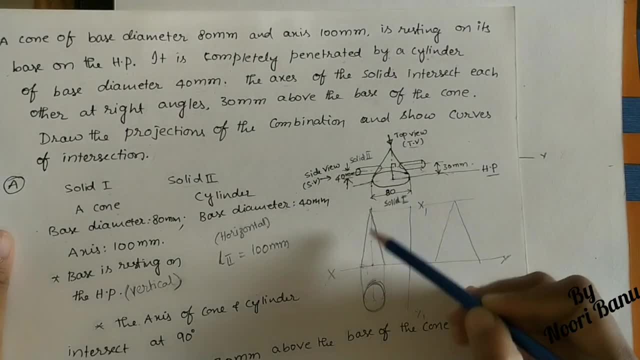 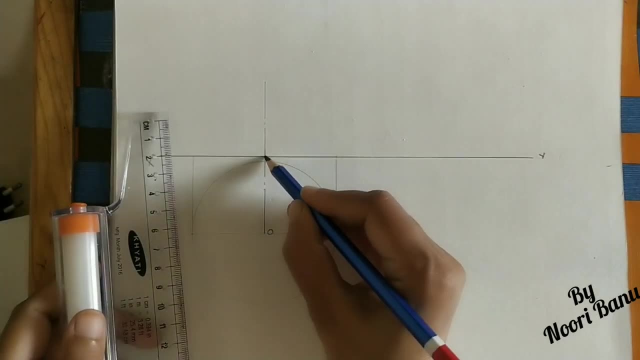 Okay, This is the top view Now. after that we will do the front view. How much height? it is 10 centimeter, Okay. So extend this axis line up to 10 centimeter. So from this point it should be 10 centimeter. 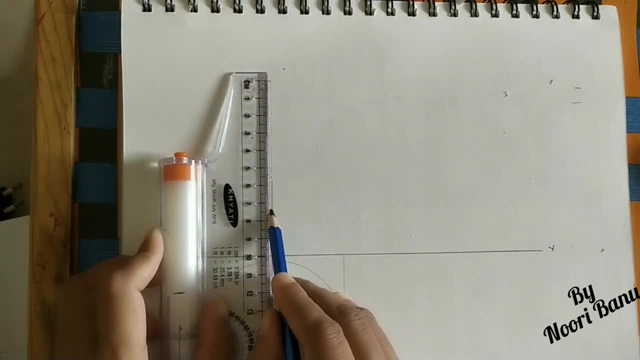 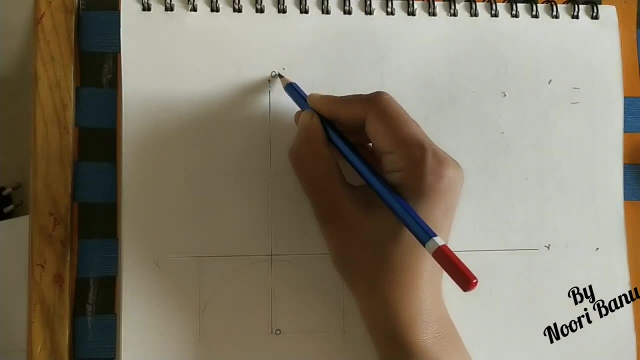 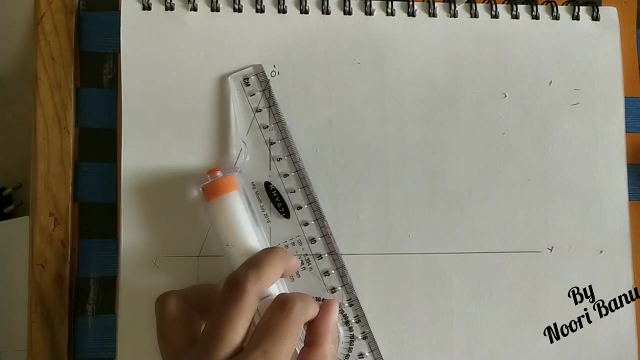 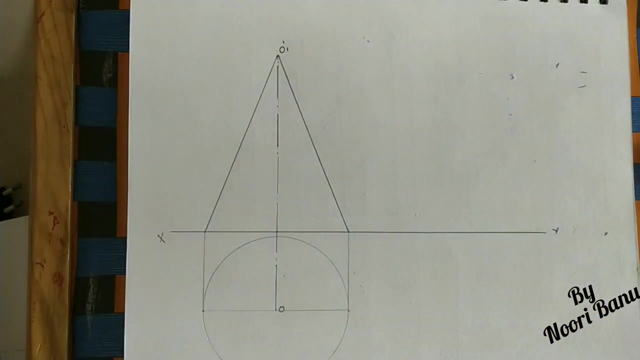 From this point, take 10 centimeter, Just extend this axis line. Now this is the apex For apex. let us take O1 dash I am taking. Okay, Join these points to this apex. This is the front view. this is the top view of the solid one. for getting the side view, just do one more reference line. 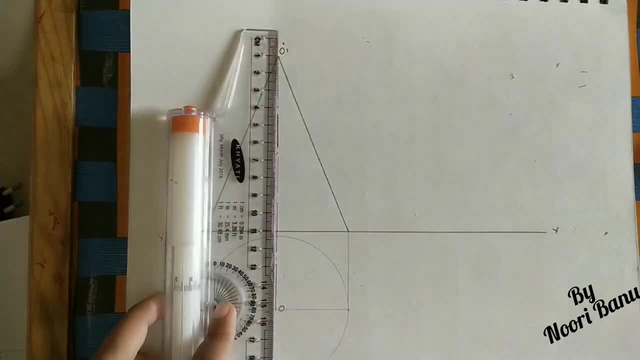 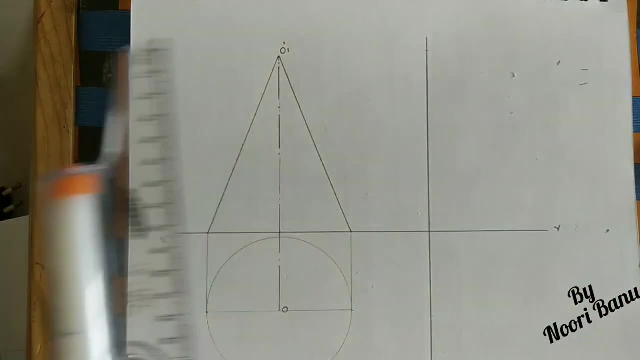 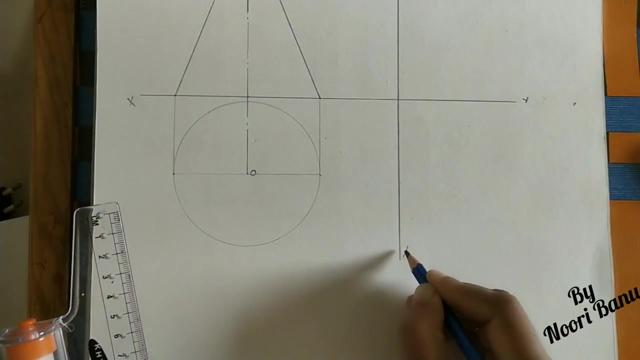 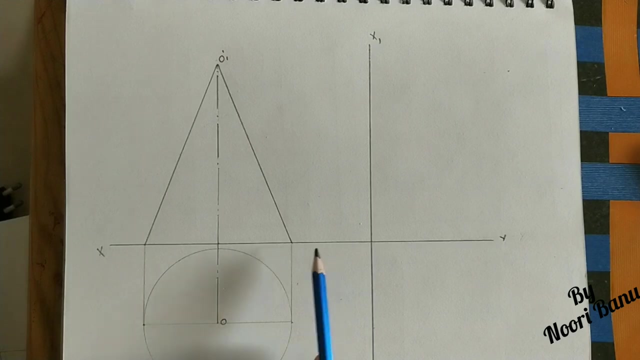 So take, this is the reference line for doing the vertical line here. Move the scale Here. take the reference line. So instead of XY I am giving X1, here Y1.. Here we will get the side view Here from all the points. do the projector line from these points. already we did the line here also, do the projector line. 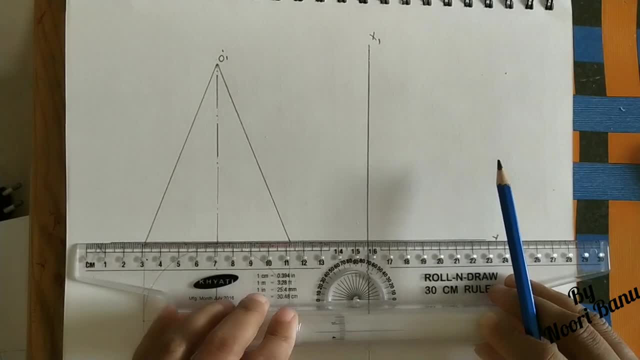 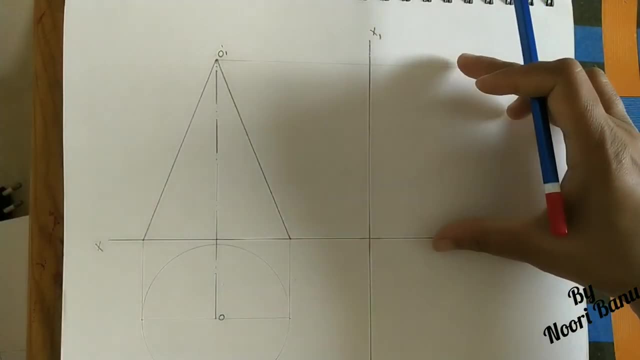 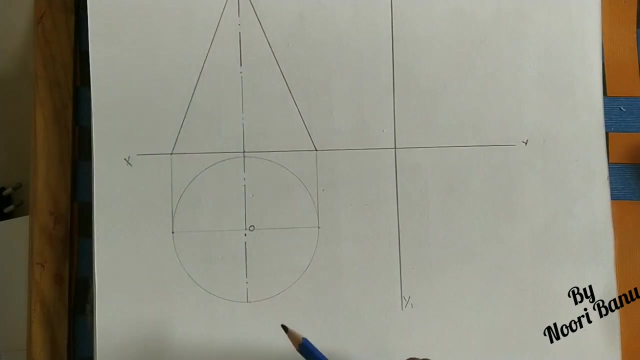 Take, this is the reference line, Move the scale, So this will indicate height of the cone in the side view also will get the same height. Okay, Extend this axis line, this side also, So from the top view, also from these points do the projector lines. 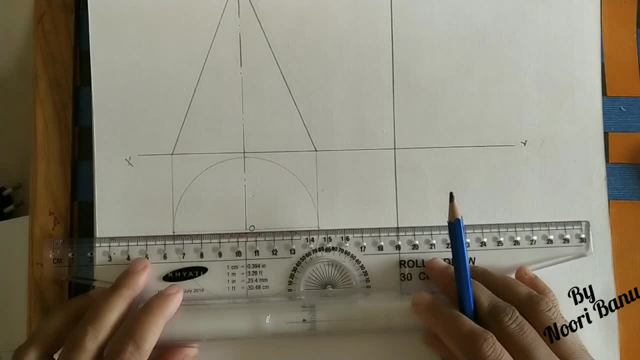 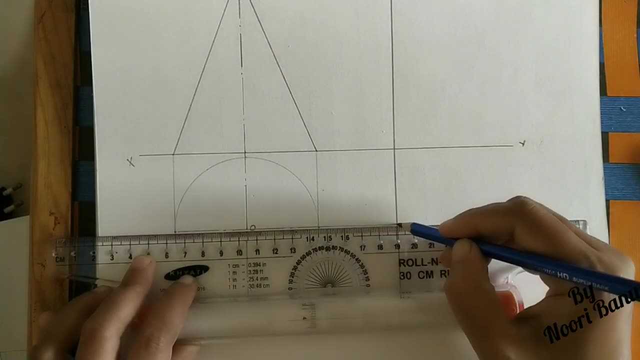 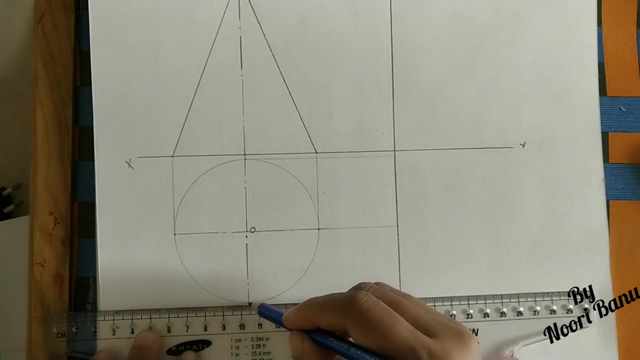 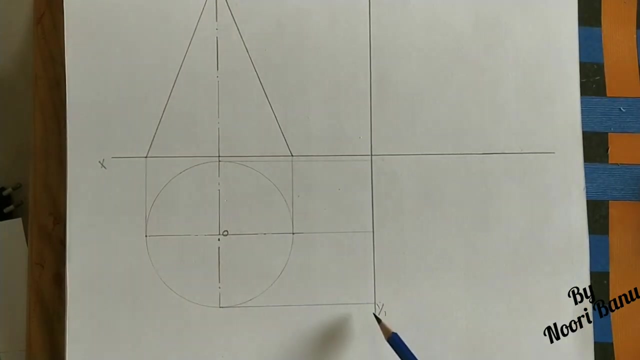 Up to this line. Take, this is the reference line. Okay, Do the axis here. Here. do the projector line Here also. do one line Here also do one line. So you will get these points on this reference line. After getting these points here, shift these points on this reference line. 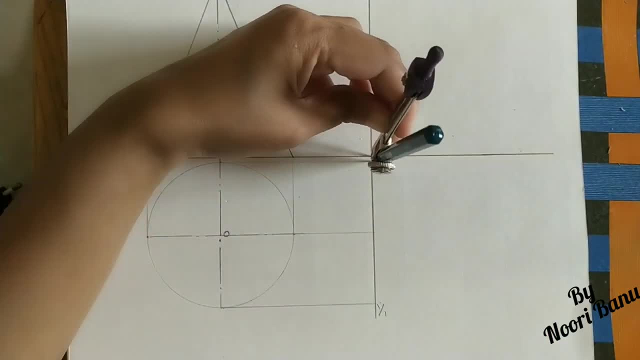 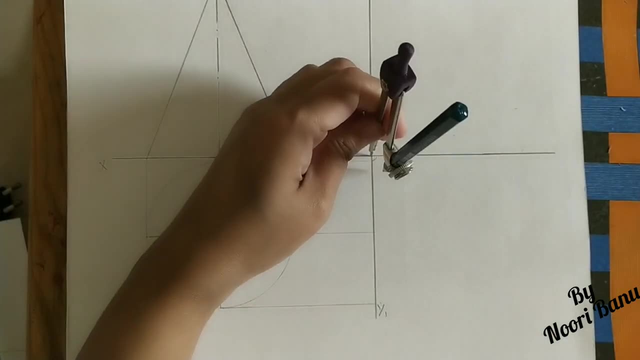 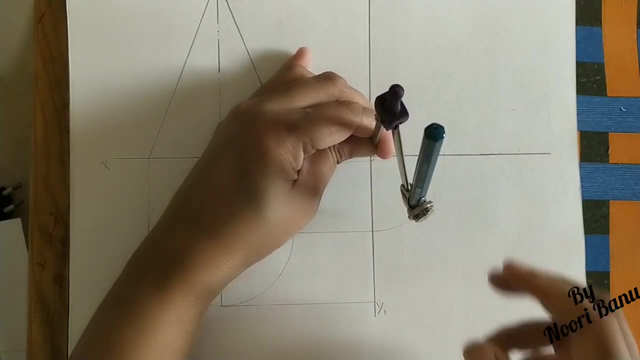 Take this point as center, This distance as radius shift to the reference line. and now take the same point as center. This length is a radius shift that point to this reference line. again, take same point as center. This length is a radius shift up to this line. 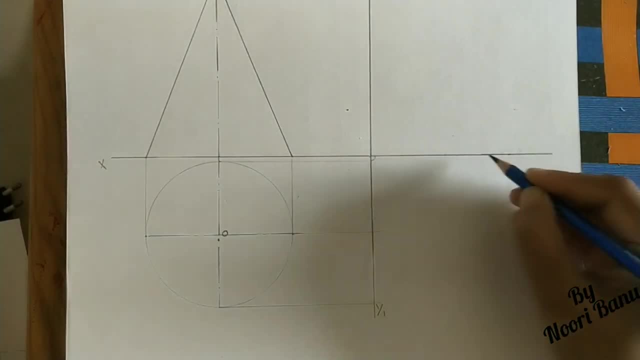 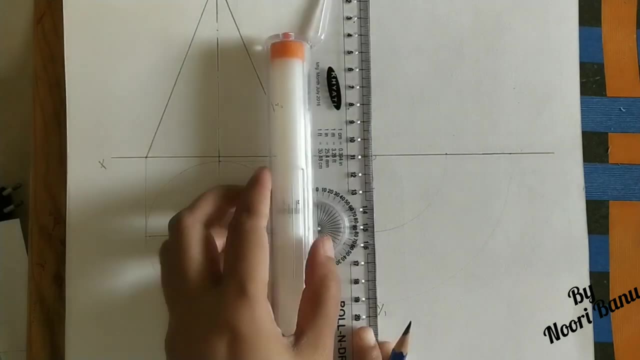 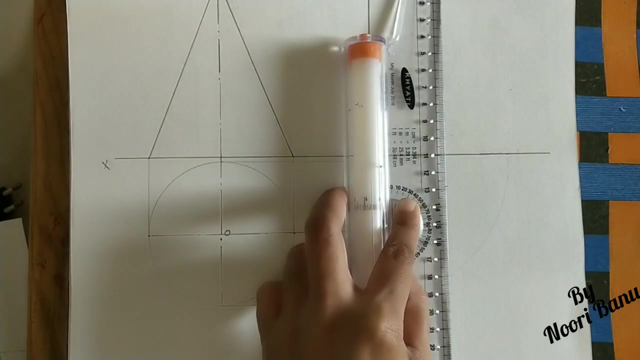 Take this intersection points Here. this is the axis line. Okay, Just do the axis here. Okay, This is the reference line. Move the scale up to this center point and do up to this projector line. As you know, this height is same as 10 centimeter. 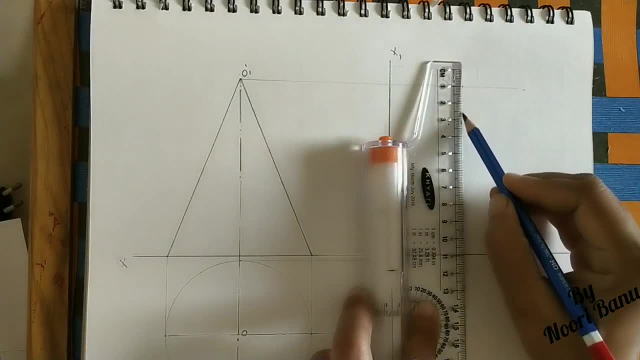 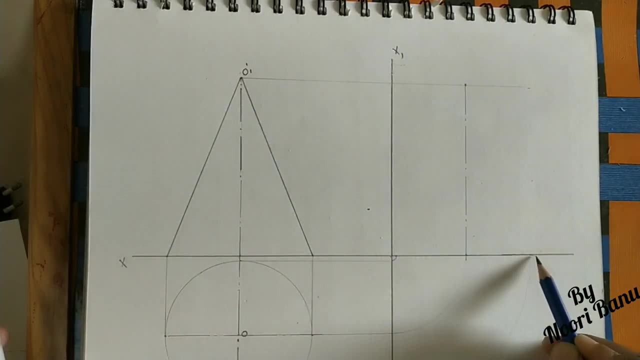 Okay, Mark this point here. on this line, projector line, Do the axis, Two big lines with the dot And take these points. Okay, Join these points to this apex For apex. I am marking. Oh, one dash here for side views. 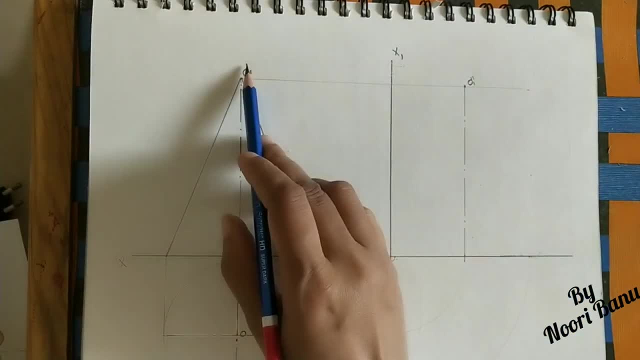 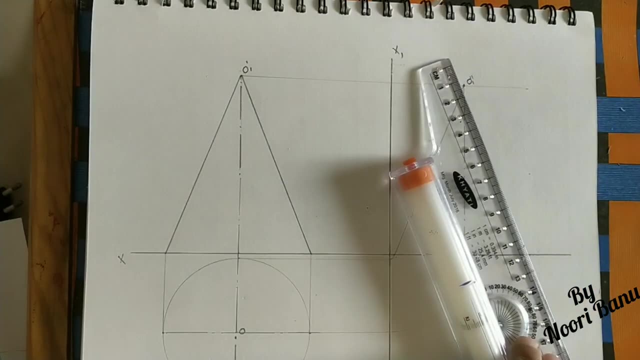 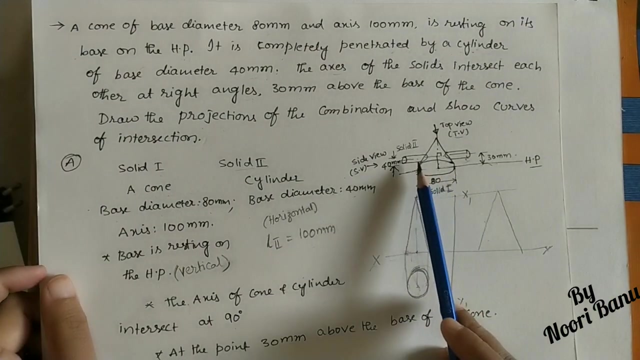 I am marking: Oh, one double dash. It's same point here. one dash here, double dash. Okay, Join these points to the apex. Now, this is the side view for the solid one. We did these three views and after that we had to do the combined three views. 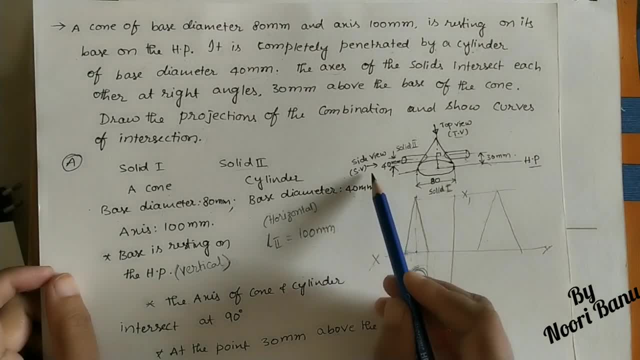 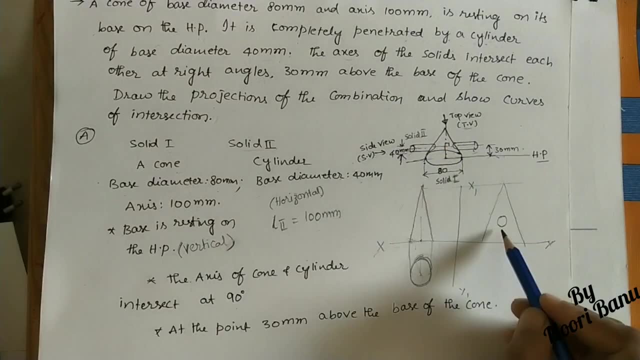 Okay, Whenever combined three views of given for the intersection of solid. initially do the side view. If you take the side view from this side, you can see this circle, Okay, on the surface of the pole. So here we can see the circle of this cylinder. 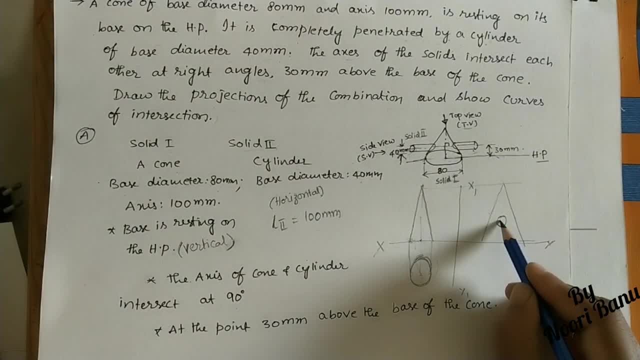 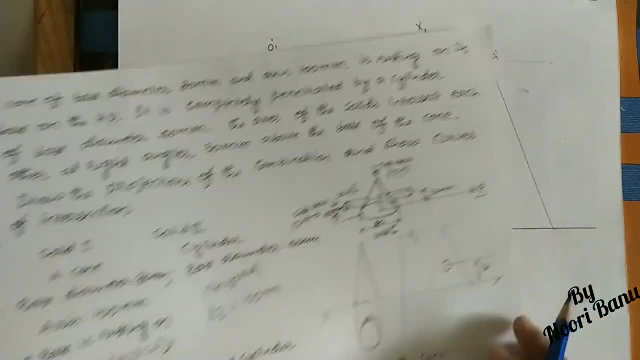 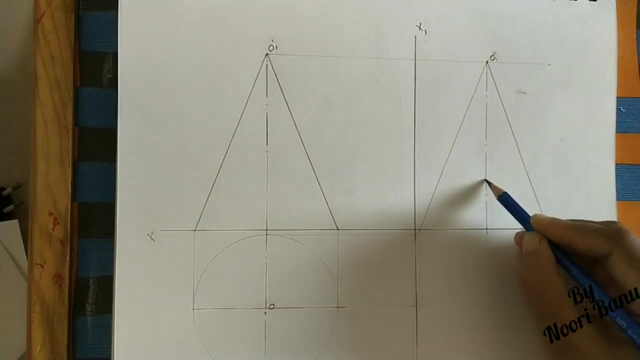 How much distance. it is 30 mm from the base. So from the base this center is 30 mm. So on the axis mark this distance 30 mm. So from here, take 3 centimeter. Here it is a center of the circle. 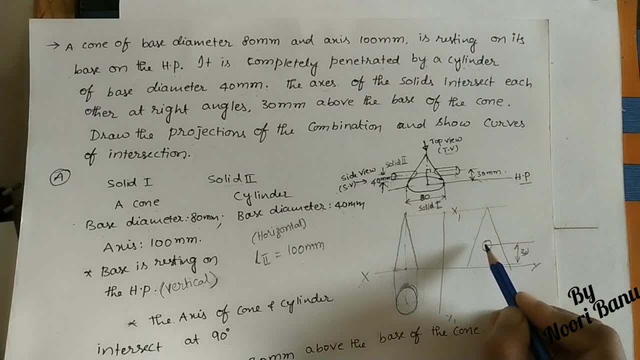 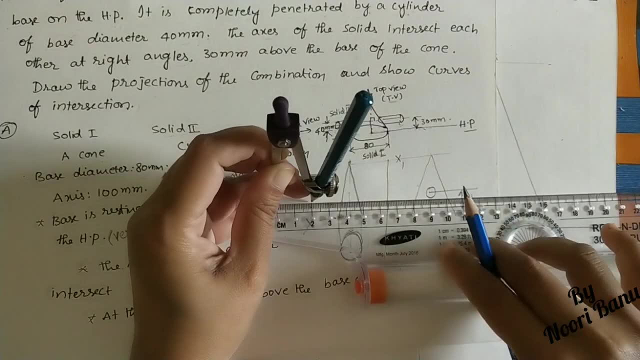 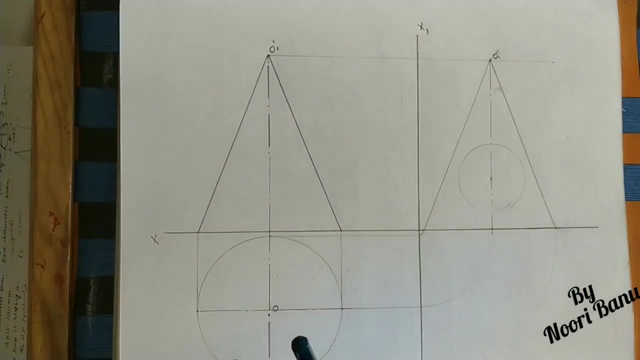 Diameter of the cylinder is 40 mm. Radius is 2 centimeter. Okay, from this center, Radius is 2 centimeter. do do a circle. 2 centimeter is the radius. So at this point, do the circle. Getting the circle divide the circle into 12 equal divisions. 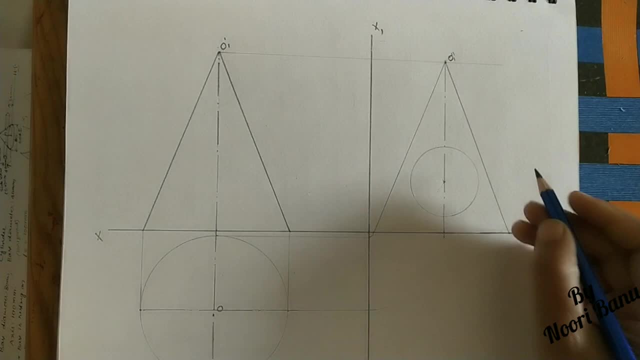 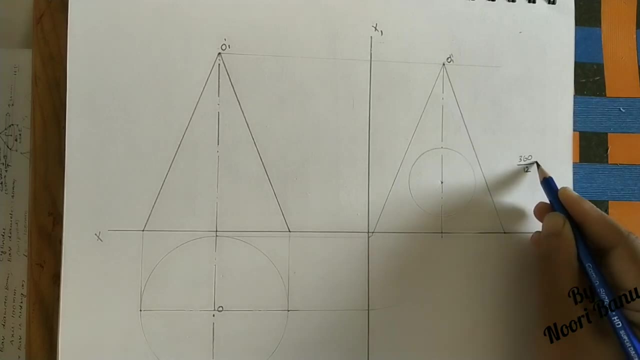 We can divide into any number of parts: 6 or 8 or 12. here I'm dividing into 12 equal divisions. So at any circle, angle at the center is 360. divide this into 12 equal divisions. Each division is 30 degrees. 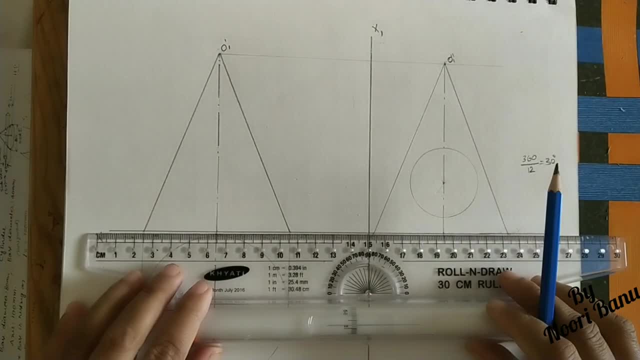 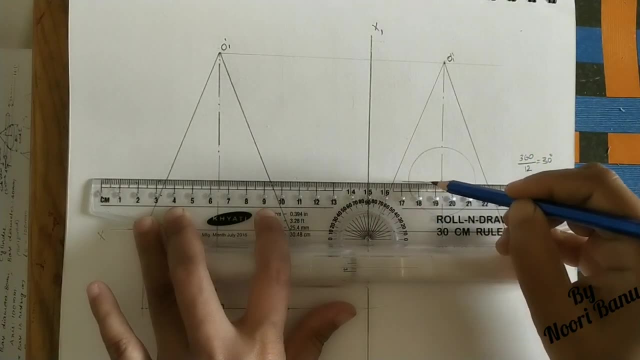 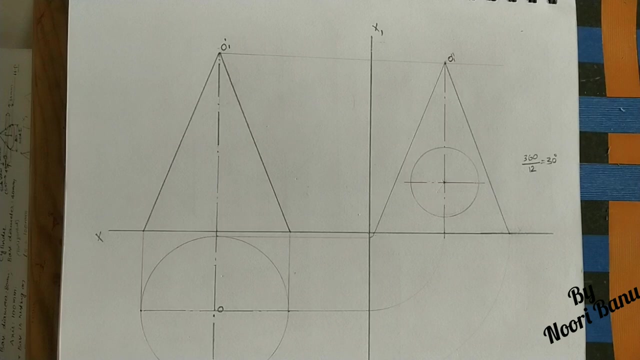 So here I will take horizontal diameter also. Take this is the reference line, Okay, from the center It is the axis line. Just do axis line here. Okay, so from this line divide 30 degrees, next 36 degrees, like that. Take this bigger diameter is the reference line. 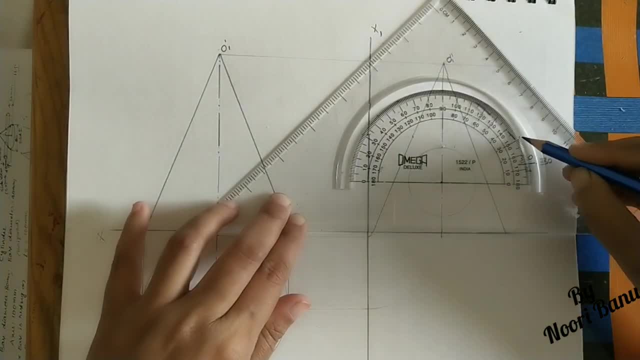 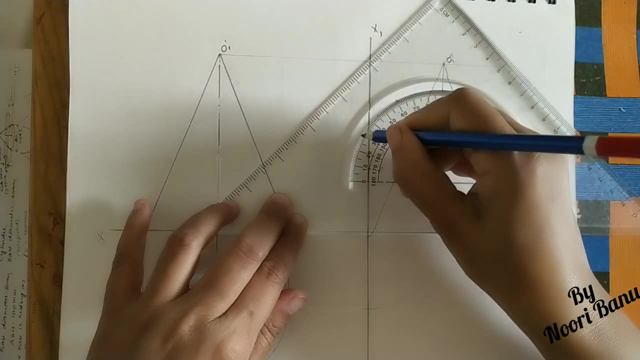 Take 30 degrees here, first part: 30, 30 plus 30.. 60, 60 plus 30 means 90, 90 plus 30 means 120. 120 plus 30 means 150. 150 plus 30 means 180.. 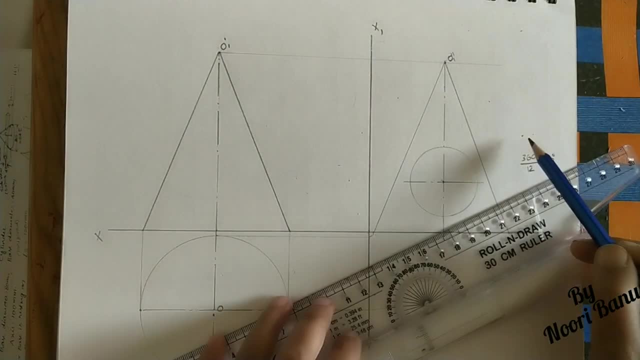 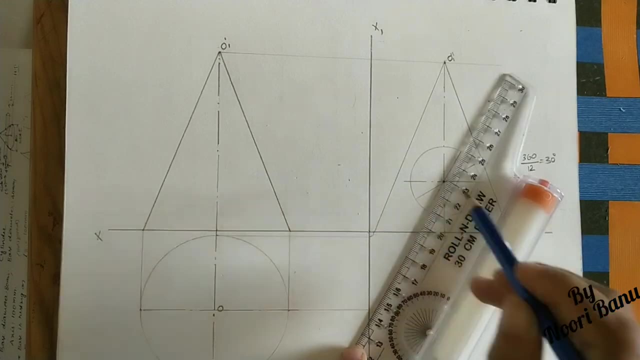 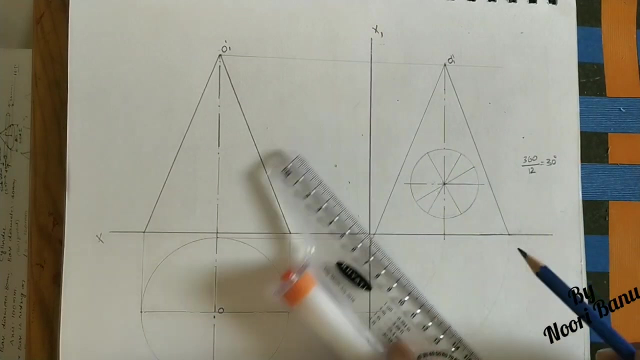 Join all these points to the center. So this is the initial point. Do the line inside the circle in this direction. Similarly, this point. Next, already we did the axis line here. Next point is this point. So this point: already we did the axis. 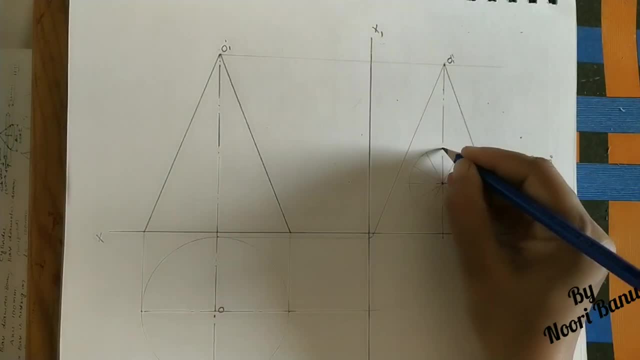 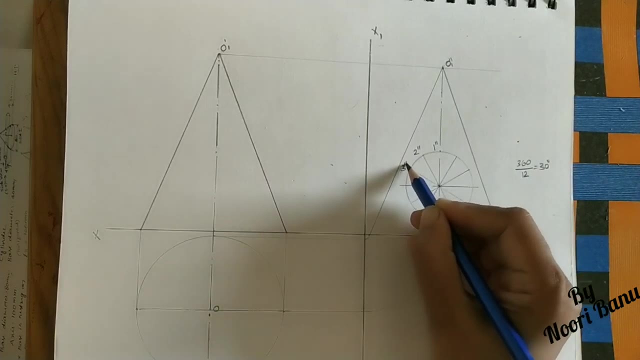 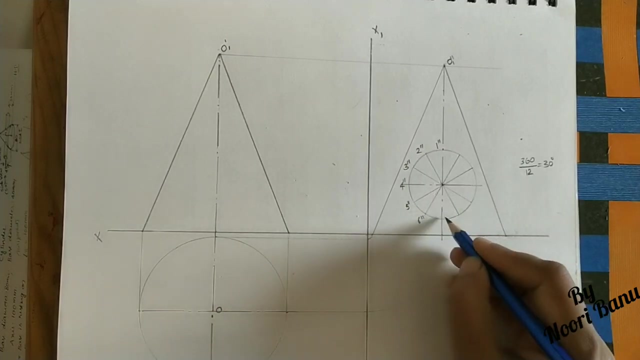 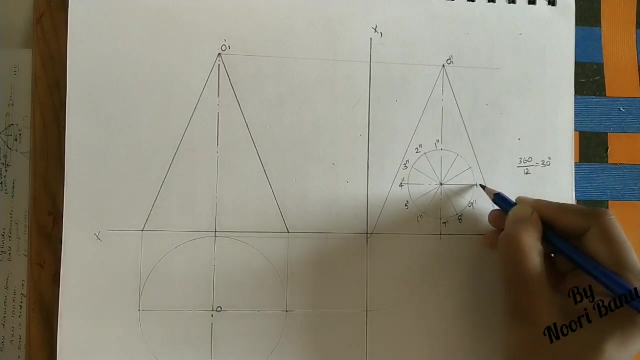 So these are the equal divisions. Do the intersection names start from this point Here? 1, double dash. I am giving 2, double dash, 3, double dash, 4, double dash, 5, double dash, 6, double dash, 7, double dash, 8, 9, 10, 11, 12.. 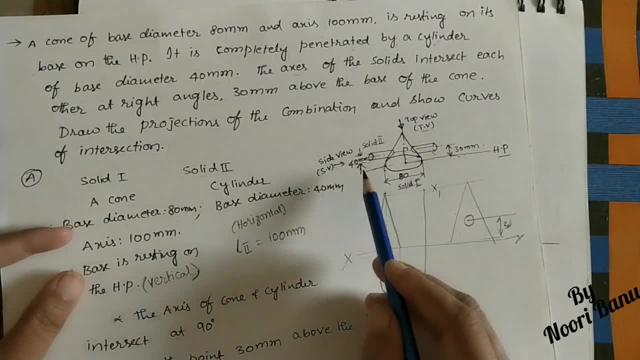 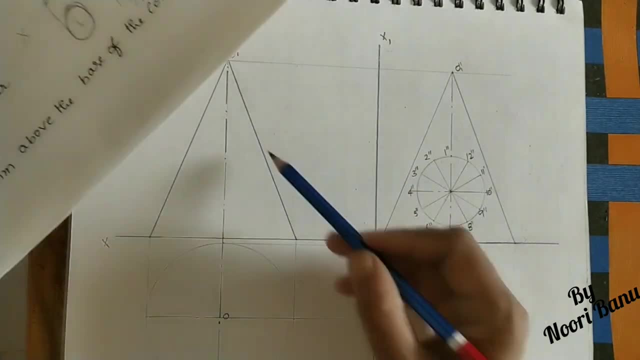 This is the side view of this combination. Okay, So after doing the side view, do the front view. Okay, in this direction. We had to see. if you see in this direction, We can see the cone already We did here. It is looking like triangle after that. 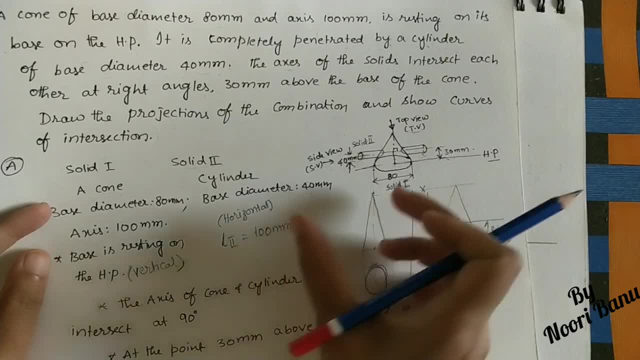 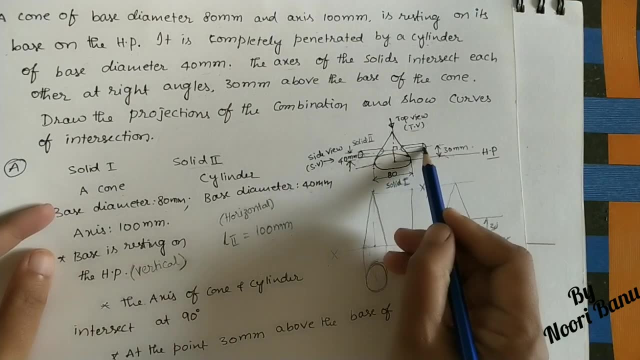 We can see this length also. Okay, total- We are assuming it is- total length is 100 mm. So this side, 50 mm from the axis, half of the length. We can see this side remaining half. We can see this side, 50 mm. first, do this cylinder. 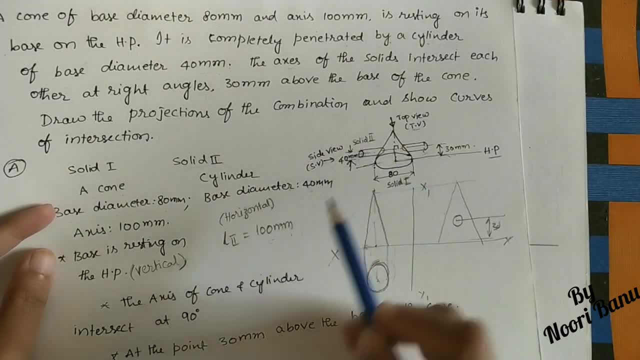 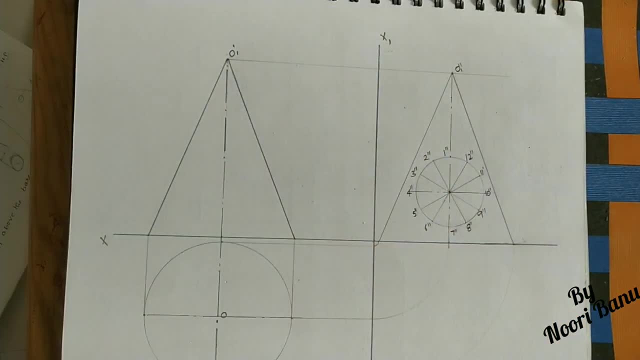 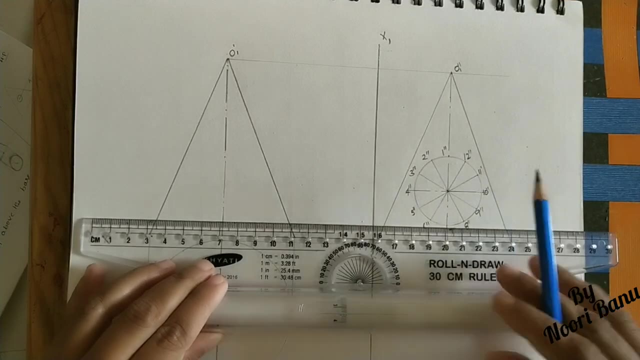 It is looking like rectangle. Okay, in this cone, first do here one box. So, whatever this diameter, we can see this same Height here. Okay, just do the projector lines from the end points. So take, this is the reference line. Do the projector line from the end points and from axis also. 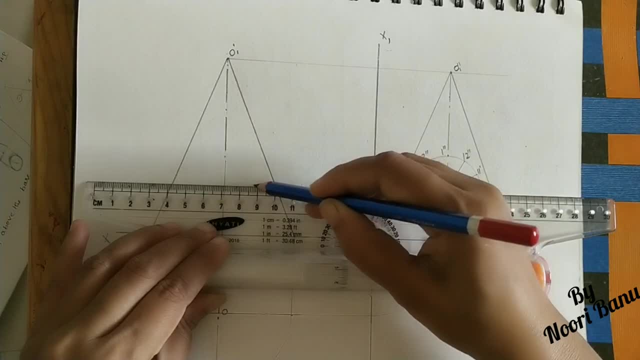 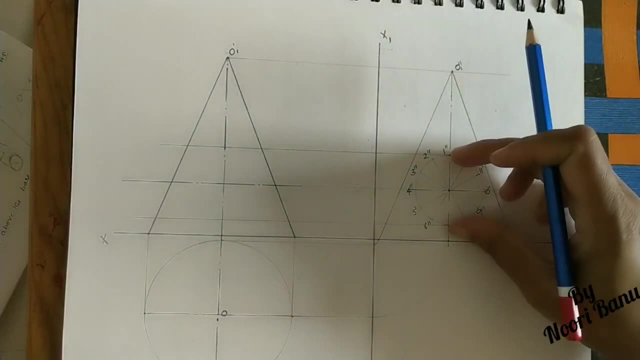 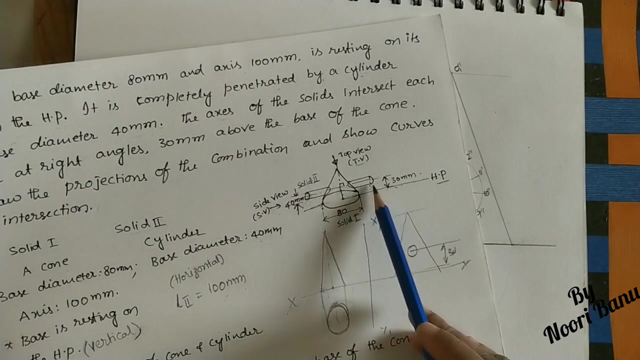 Do the projector line, here do the axis line, Two big lines with it out up to some length. Okay, and here also do the projector line. So I took the entire height. It is nothing but 40 mm I took here. So in the front view on the axis line mark this side 5 cm. 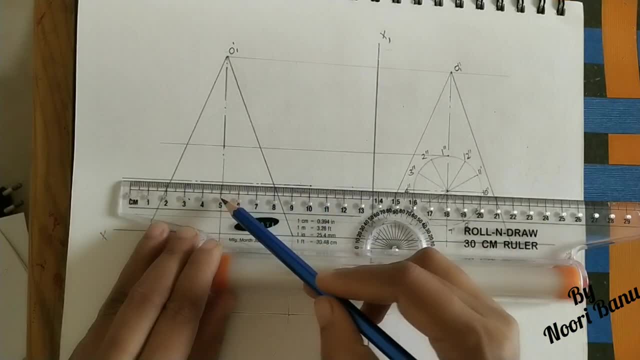 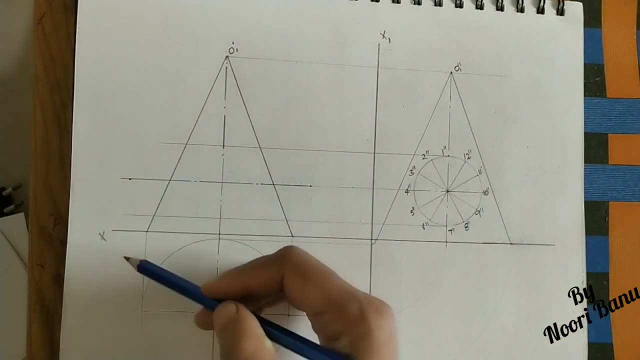 This side 5 cm on the axis line. here I'm taking 5 cm. this side, 5 cm. mark the end point here. Mark one more point here: Okay, this is the length of the cylinder. here Just do the lines like this: 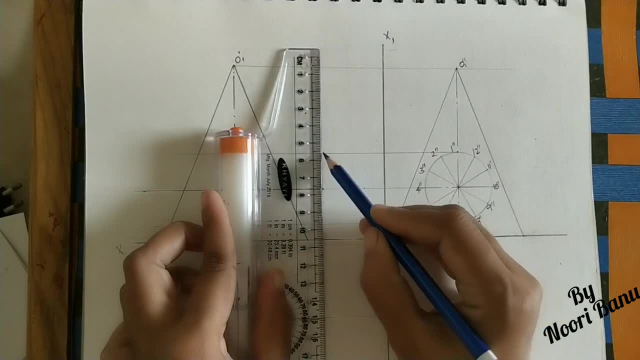 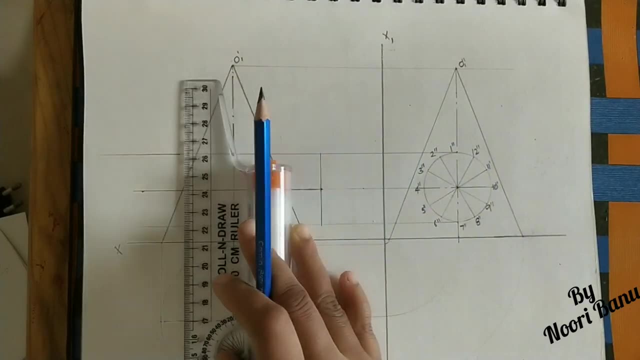 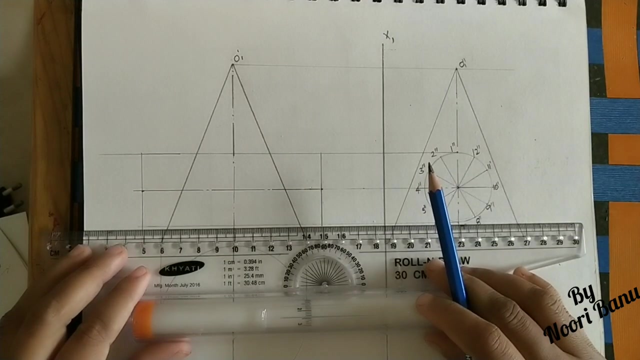 Take: this is the reference line. Move the scale up to this point. Do the vertical line. So at this point also do the vertical line. Just make it dark. So this is outside part. That's why continuous line. So this part is coming inside the cone. 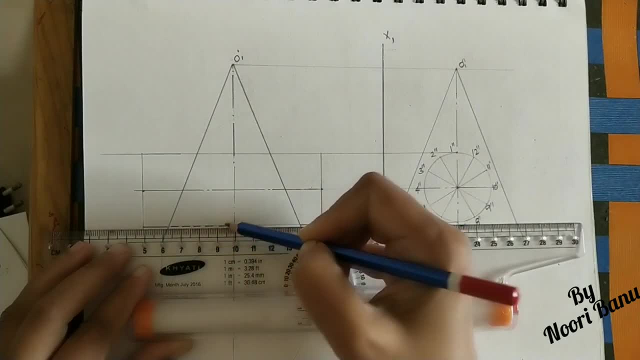 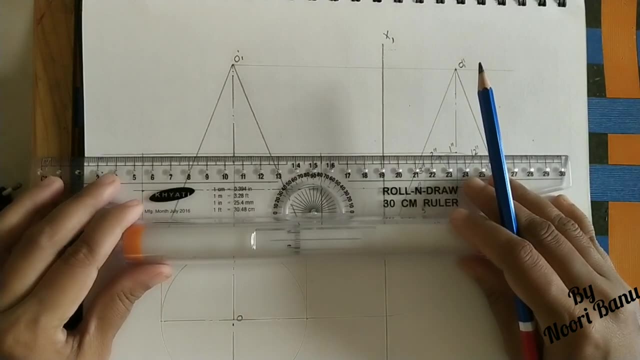 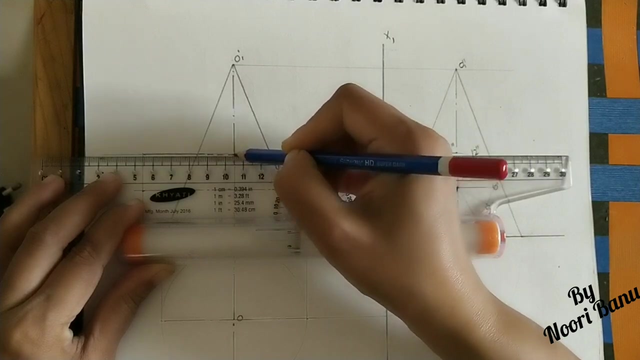 That's why it is invisible. It is dotted for invisible lines. We are doing the dashed line Like this. So here also Make this part and outside part. This part should be continuous line here. This is the invisible part With the dashed line here after intersection: 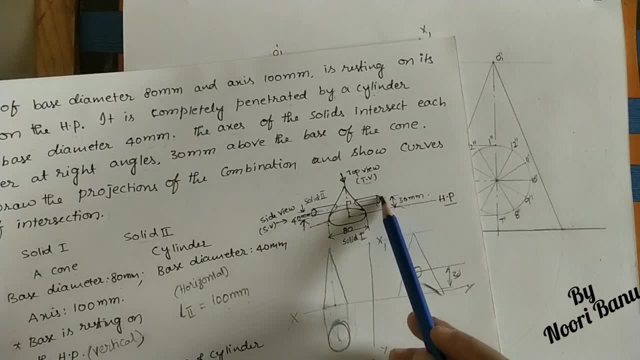 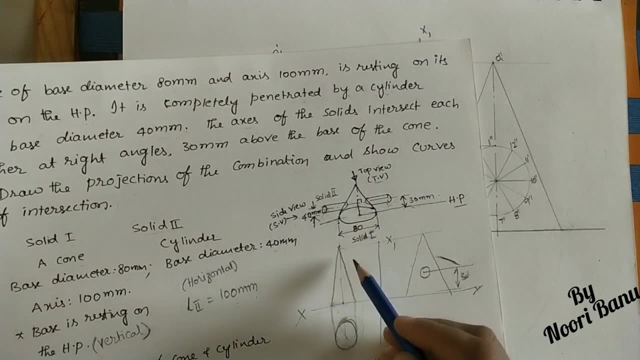 The front view is looking like this triangle and these boxes, This triangle and this boxes. Okay, this is a friend view, and similarly do in the top view also. Okay, already we did the cone circle here, So from the top view also we can see this rectangles. 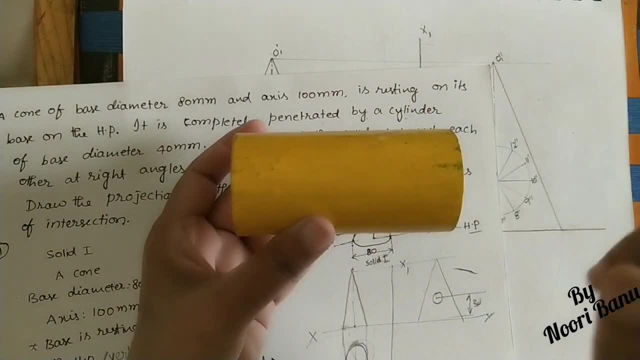 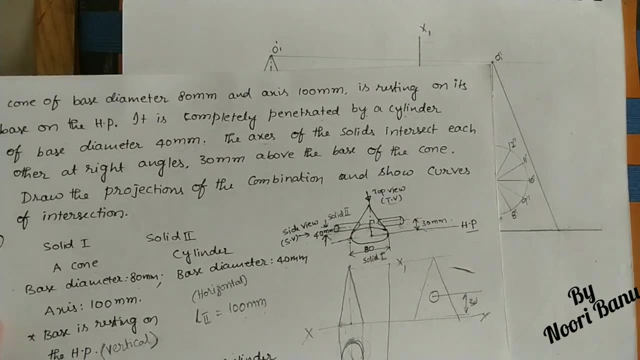 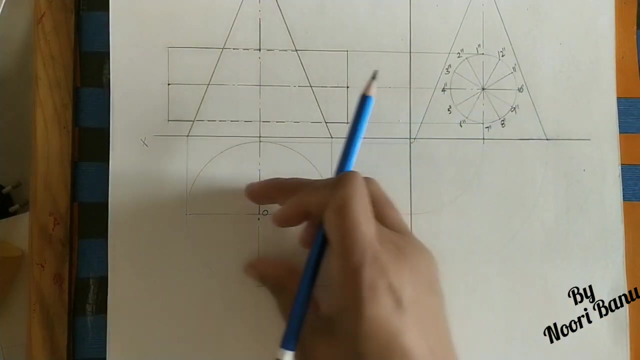 Because if you see the top view in the cylinder, it is looking like rectangle: This side, half, this side, half from the axis. Okay, it is also 5 cm And 5 cm. So here let us do the top view. Whatever this diameter, take the diameter and extend it in the top view. 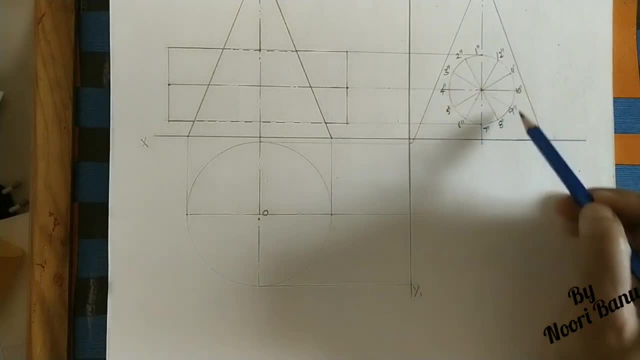 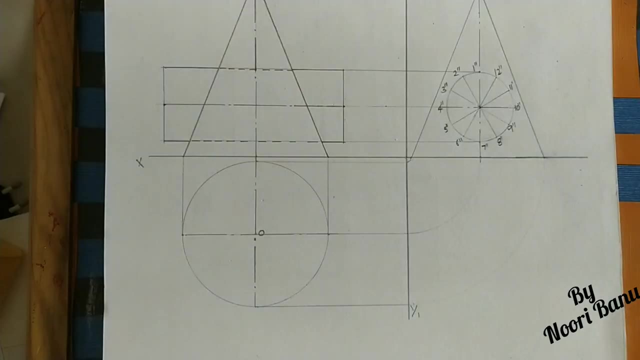 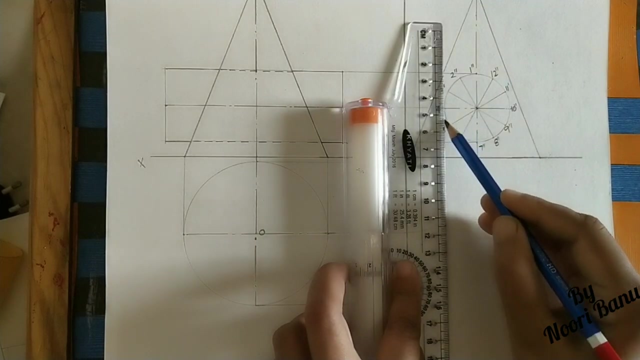 Okay, so take the horizontal diameter at these points. Do the projector lines up to this reference line. Okay, similarly, here we took the vertical. here I'm taking the horizontal projector lines. Take, this is a reference line. Move the scale, Do the projector line. 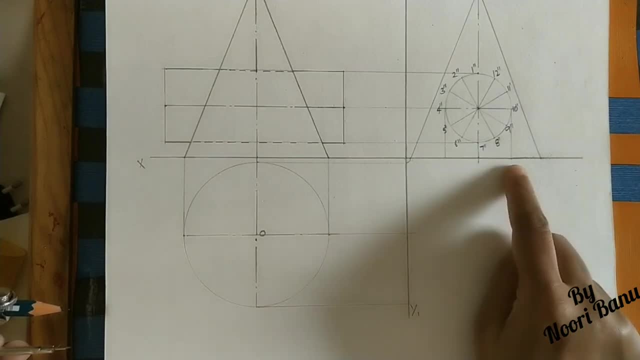 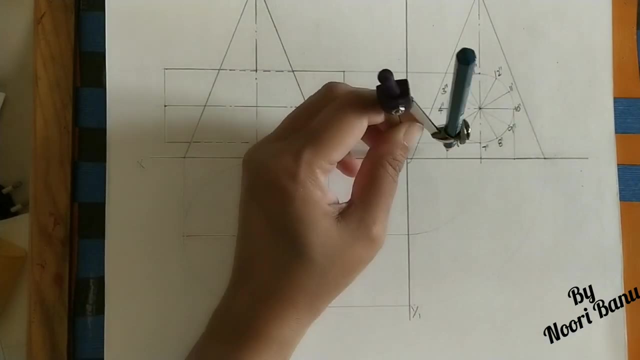 Similarly Here. also do the projector line. Shift these points. Do this: 6 y line, Already axis line. we did previously. Now shift these points. Take this point as center by using compass. This length is the radius. Shift it into this line. 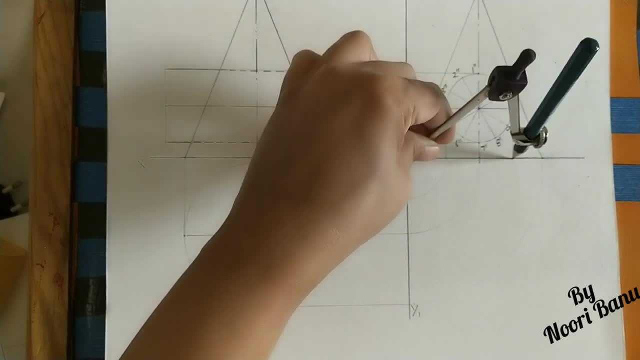 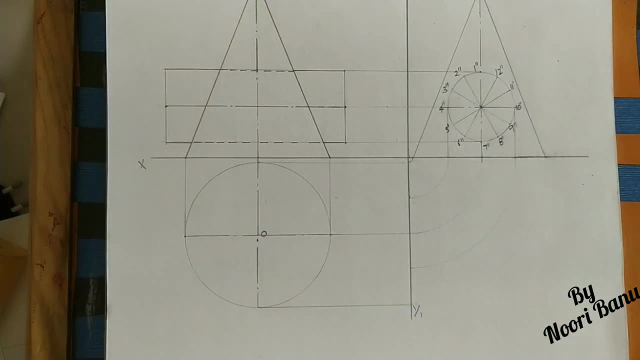 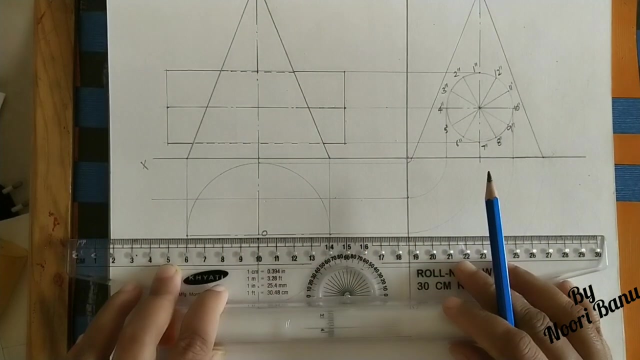 Now shift the next point. Take this length as radius, Same point as center. Now, at these points, do the projector lines? Shift this point Ready for axis? we did the line, just extend this line. so, as I told, from axis, take 5 cm. 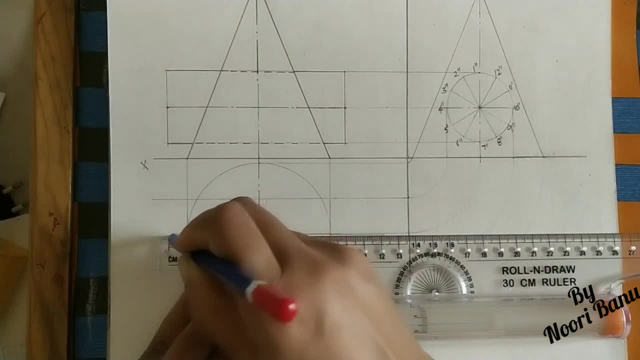 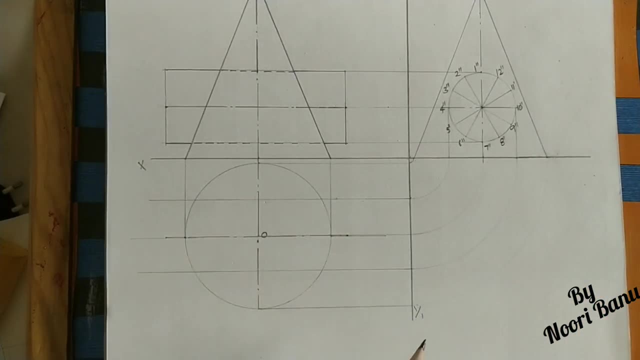 This side 5 cm. So at 5 I took this side starting point and this end 10 cm. Okay, this is the length of the cylinder in the top view. Now, these are the end points. Do the vertical lines that these points? 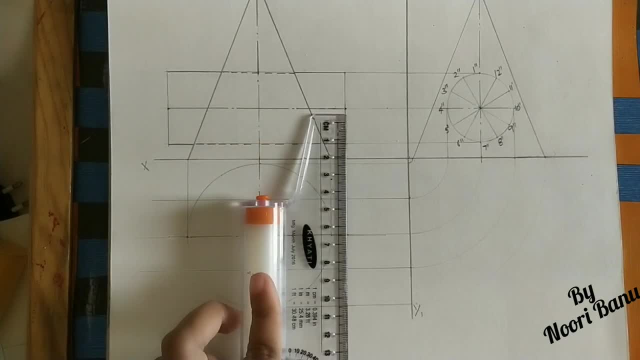 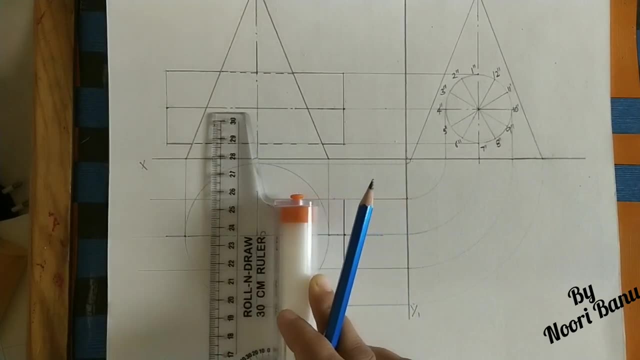 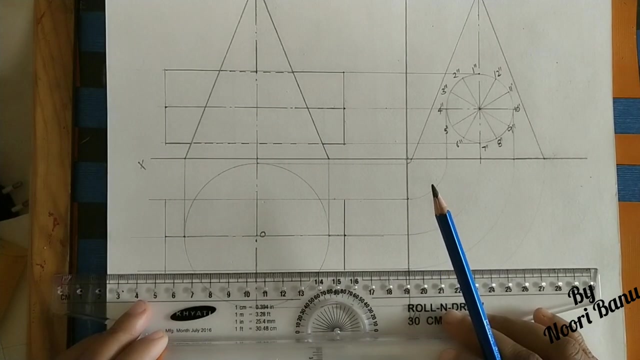 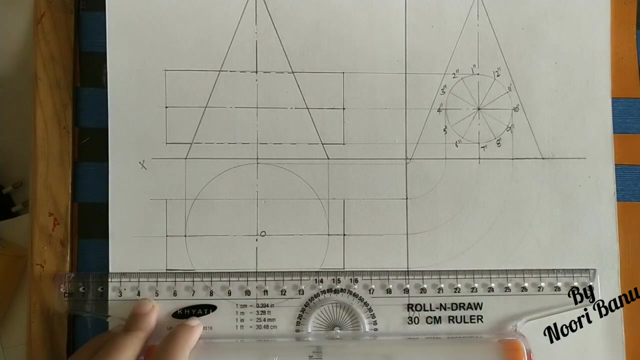 Take, this is the reference line. Make it arc line. Make it arc line. This is the axis here. also, do the lines Here, do the dark lines. Whatever outside part, it is a continuous line. The remaining is coming inside the cone. that's why it is a dotted line. Invisible part is: 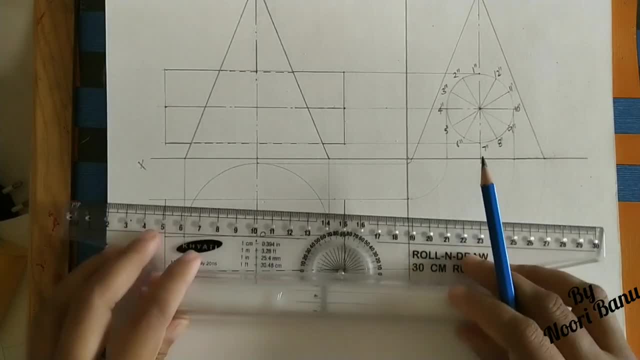 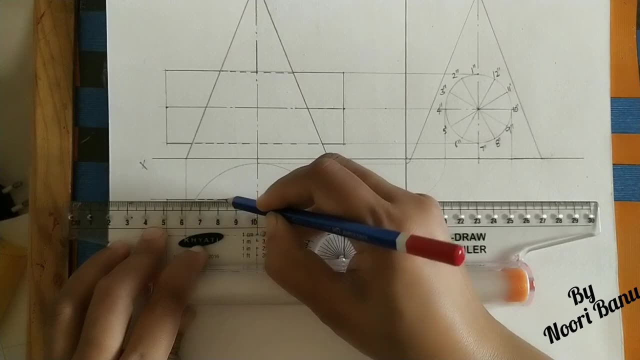 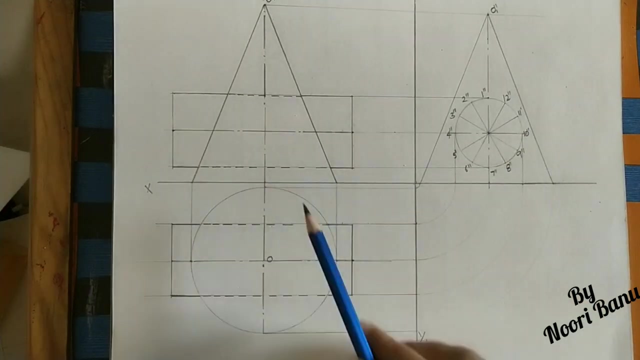 with dashed line Now here. also make the outer lines dark Inside. do the dashed line. Combined top view: This is the front view. This is the side view. Getting these 3 views Here if you take the combined side view. we have created some points on the cylinder. So, mark. 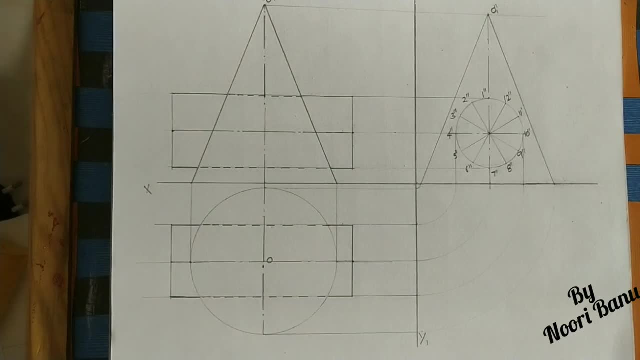 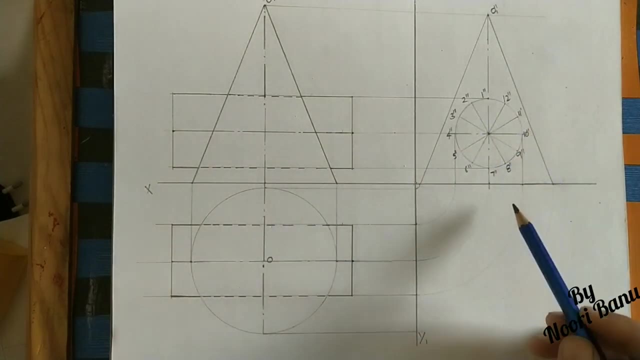 these points in the front view of the cylinder and top view of the cylinder also. So from all the points Do the projector lines in the front view as well as do the projector lines in the top view. Initially we will do the projector lines in the front view from all the points. Take. 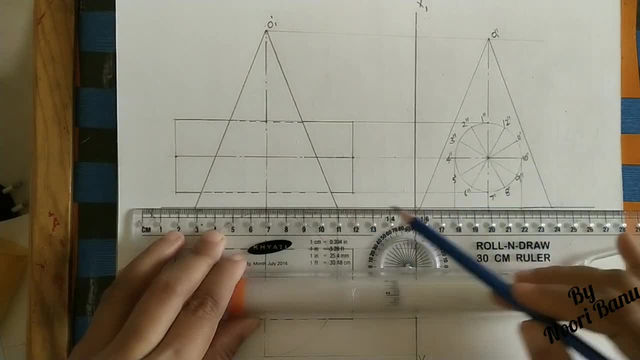 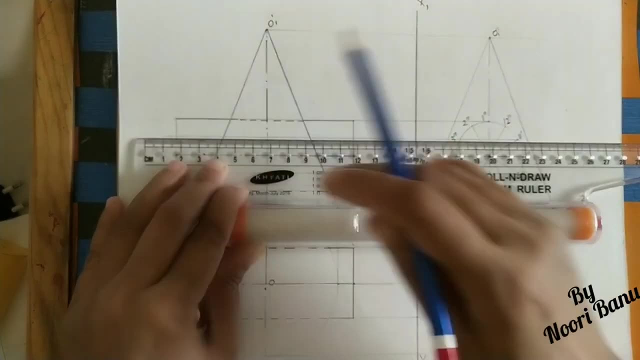 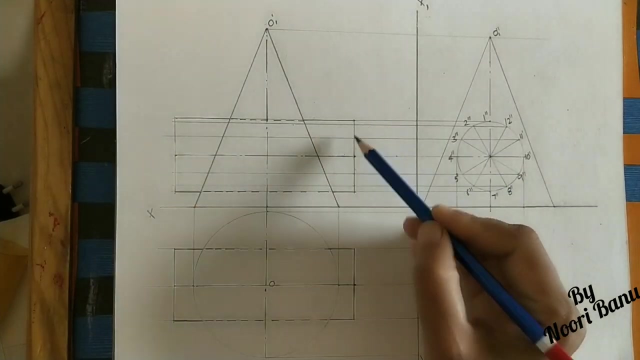 this is the reference line. Already from 7 we did the line From 6 and 8. one line is passing. We did the line. Now here mark these points on these 2 circular faces. This is a cylinder, Here one circle and here one circle. 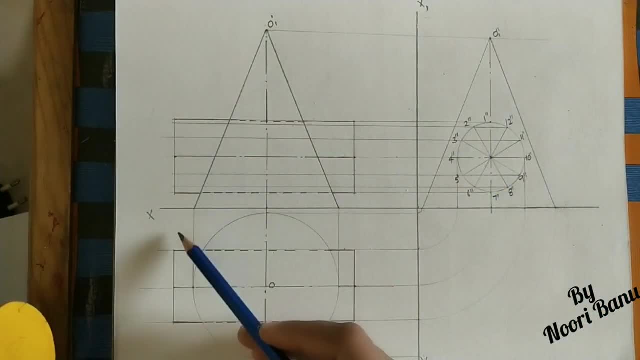 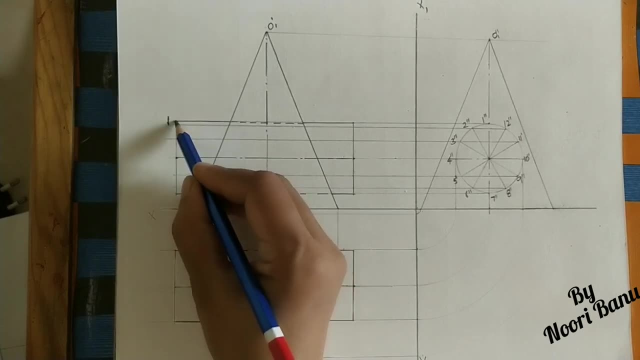 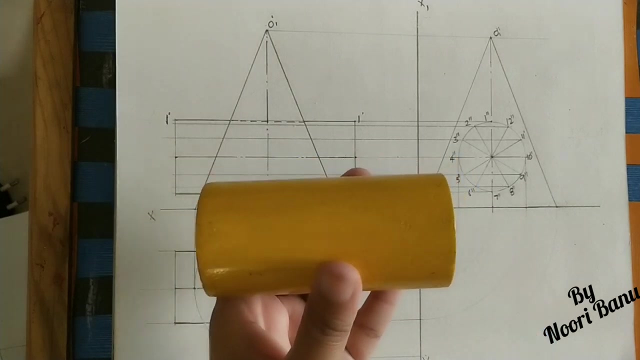 Here, this one and this one, and mark these points on these two faces. Here let us mark: 1.. this corner is one dash and let us mark this corner is one dash. This one corner is also one dash Here. 1. This surface also. i am giving one 1, one two and two like that. 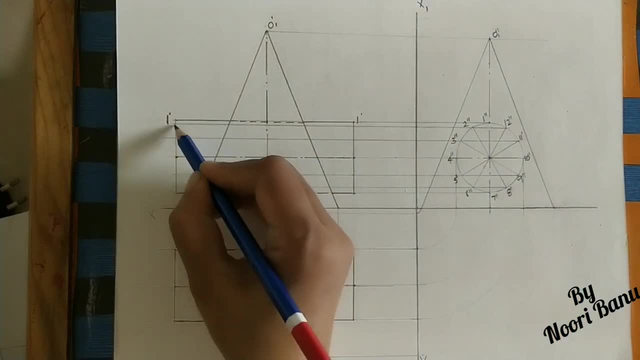 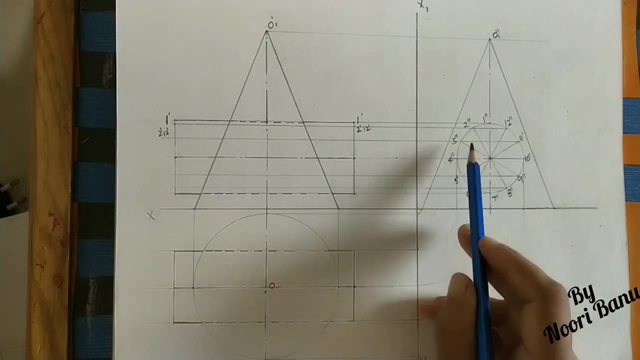 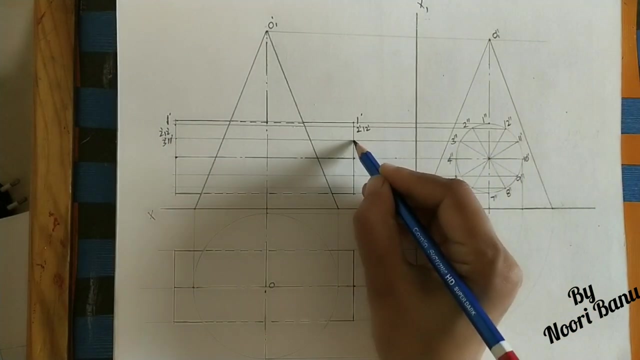 OK, after 1, two twelve line. Mark these points: two dash, twelve-dash. Here also two dash. twelve-dash, 11 dash, 3, 11, 3 dash, 11 dash. here also 3 dash, 11 dash. after 3, 11, next 4 and 10. okay, here 4 dash. 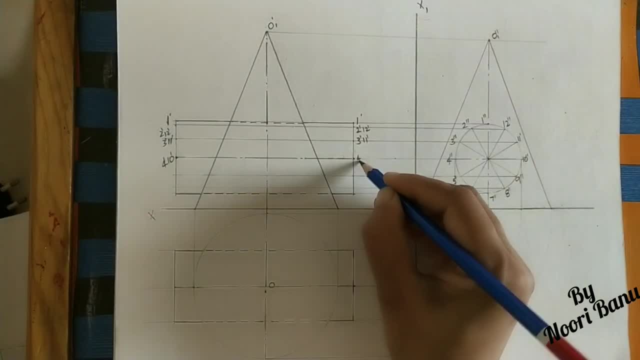 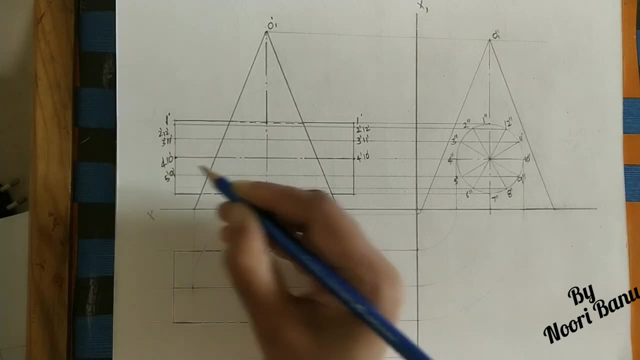 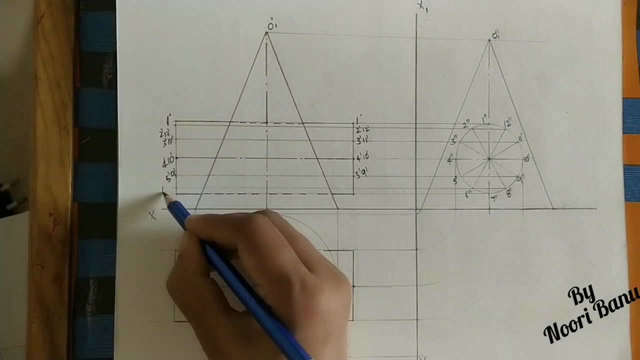 10 dash here. 4 dash 10 dash after 4: 10. next 5, 9 here. 5 dash 9 dash here. 5 dash 9 dash next after 5, 9, 6, 8. okay. next point is 6 dash 8 dash here. also 6 dash 8 dash. next point is 7. 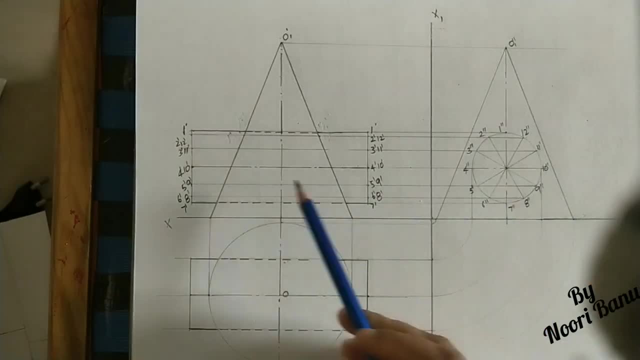 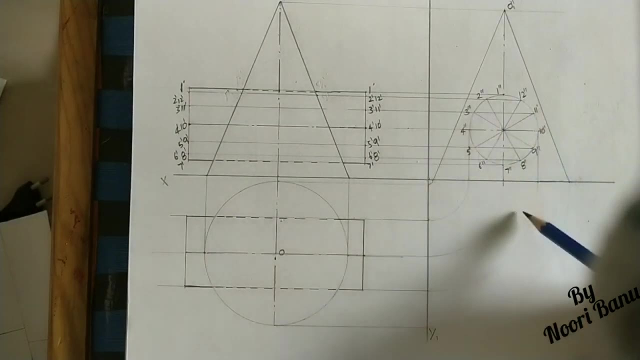 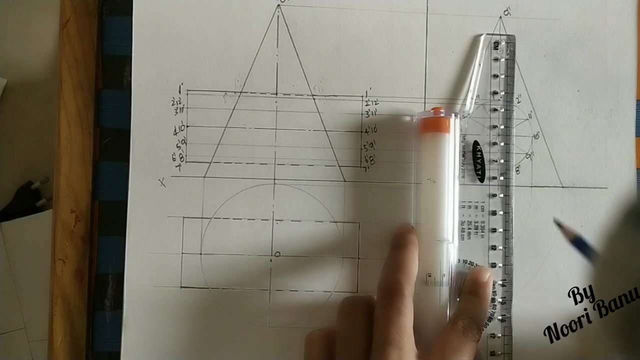 here: mark 7 dash. here also 7 dash. after marking all the points in the front view, mark these points in the top view also, for doing it, do the projector lines from all the points up to this reference line take. this line is a reference line and at 12 and 8, 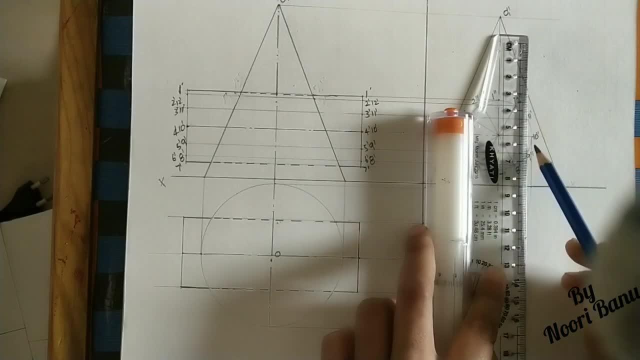 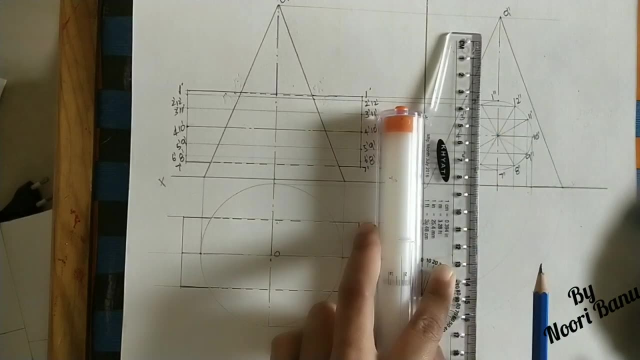 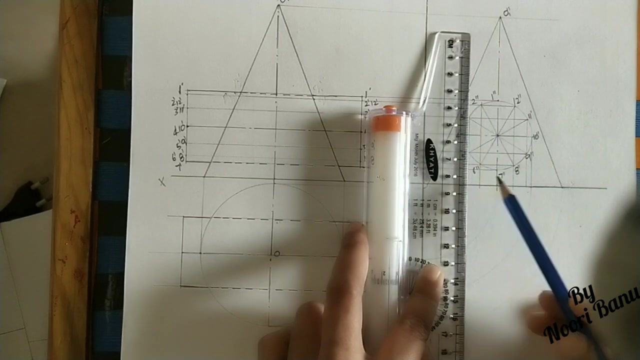 one line is coming: 11 and 9.. From 10: already we took the line Mark this side also. From 2 and 6.. 3 and 5.. And already we took the line at 4 end point. Okay, shift all these. 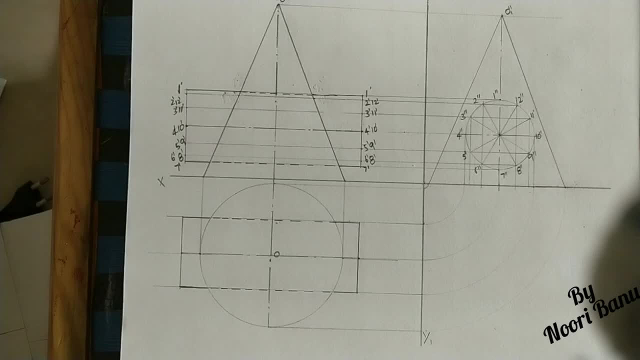 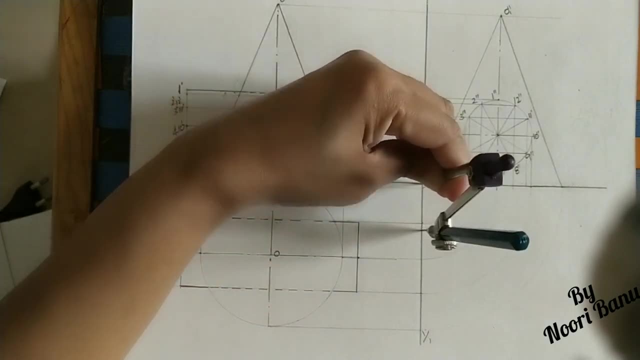 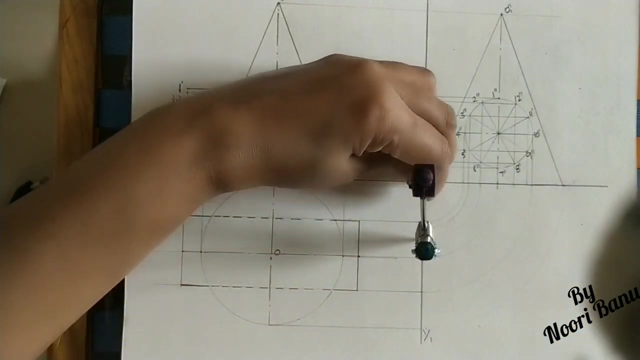 points to this reference line by using the compass. Take this point as center. Take this is the radius. Shift it into this reference line. After this point, take the next point, Same point as center. Shift it into this reference line. Now axis line. already we did previously. 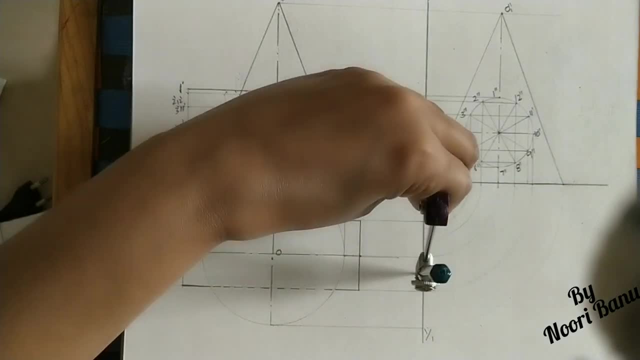 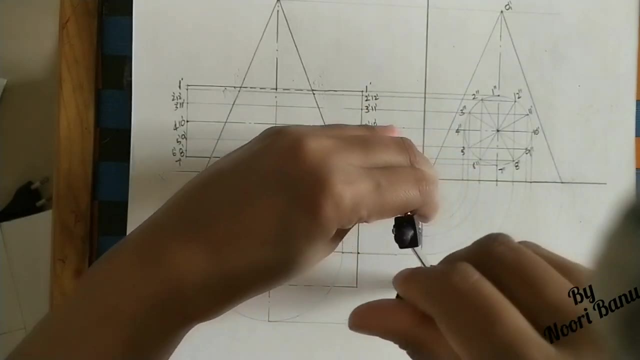 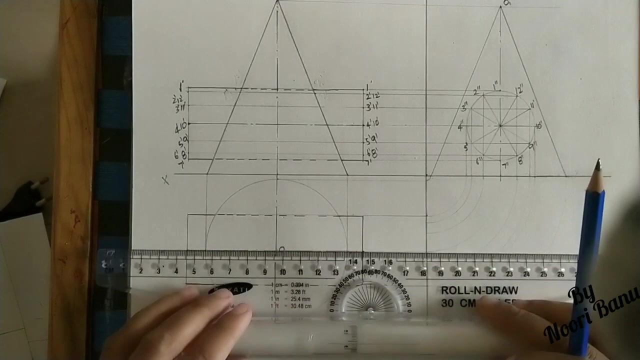 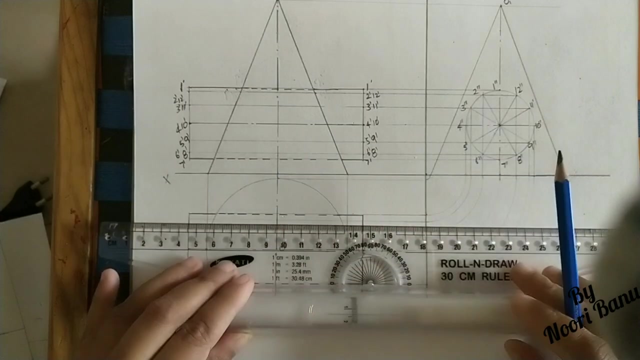 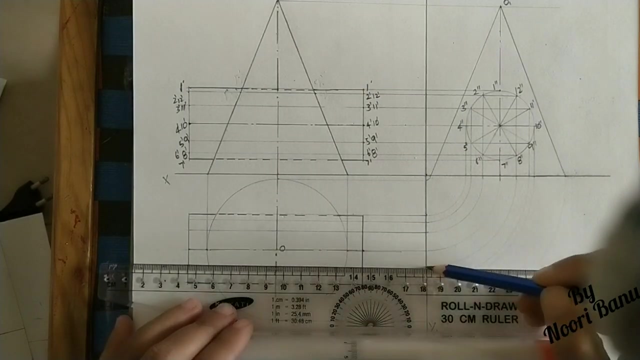 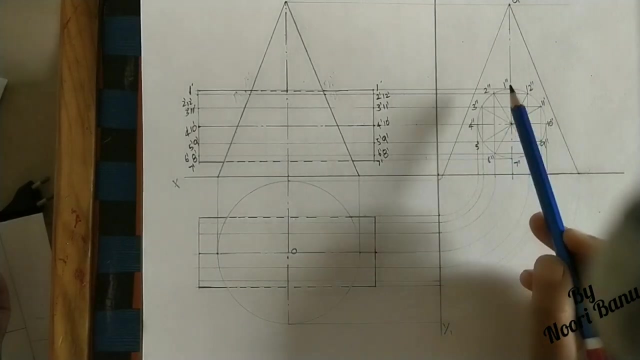 Next point is this one: Take this length, Shift it into this line. After this, take this point, Take this length, Shift it here. From all these points, do the projector lines inside this cylinder? Okay, This is the reference line Getting the projector lines. mark these points, Okay. 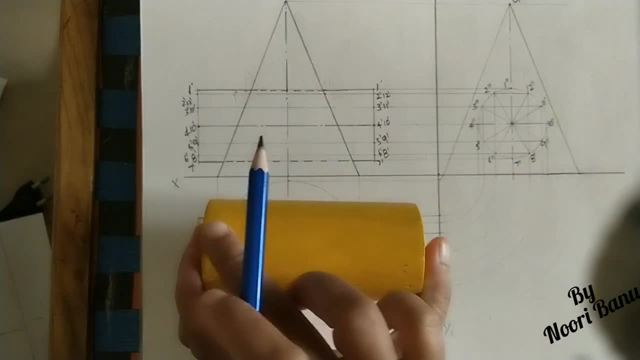 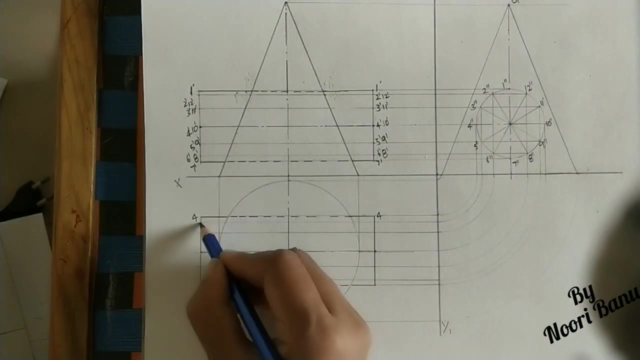 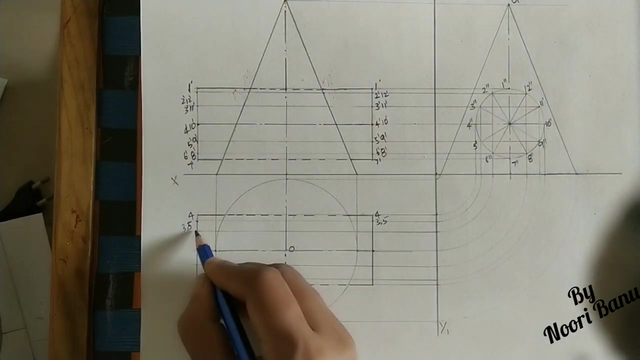 So first initial point is 4.. So at both sides of the cylinder we are marking 4 comma 4 here, Next 3, 5.. Okay, So this point is 3 comma 5.. Here it is 3 comma 5.. Next 2 comma 6.. Next. 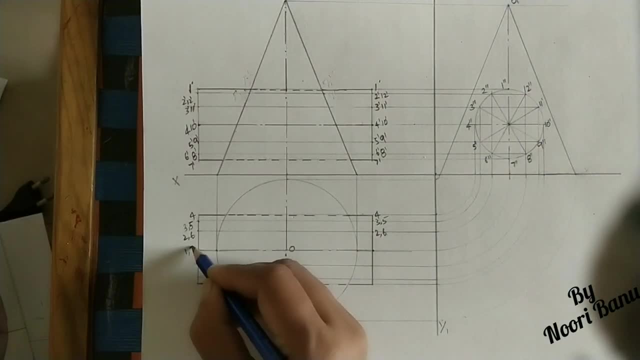 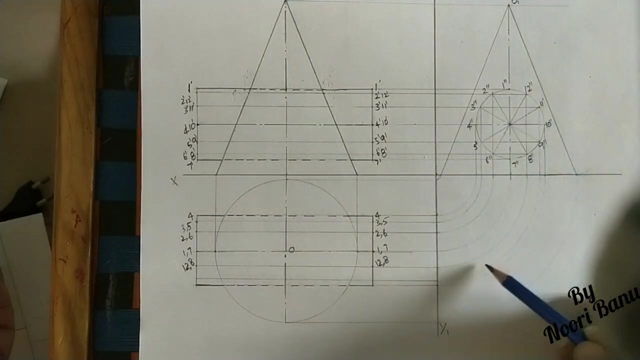 point 1, comma 7.. Next, after 1: 7, next 12, 8.. After 12: 8, take 11, 9.. After 11: 9, take 10.. So we have marked all the points in the front view as well as in the top view. After getting, this is the combined front view combined. 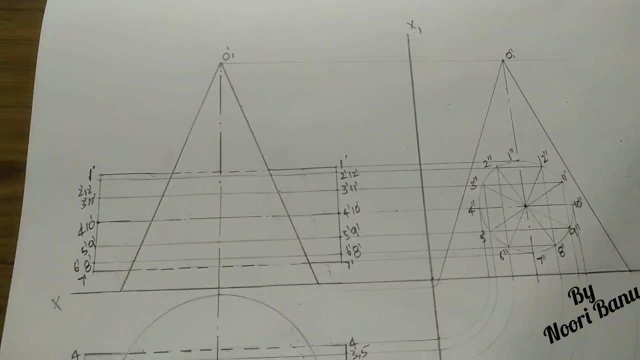 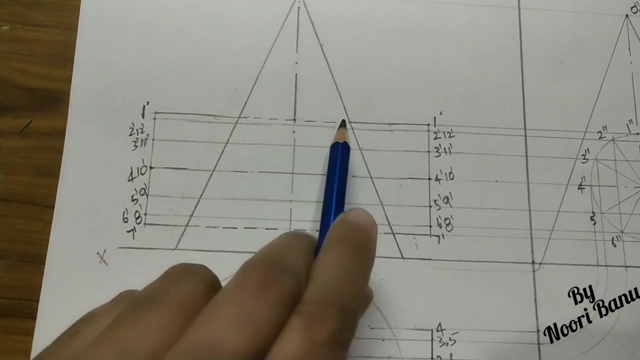 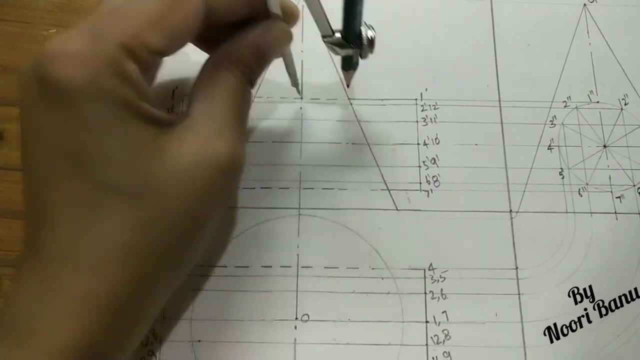 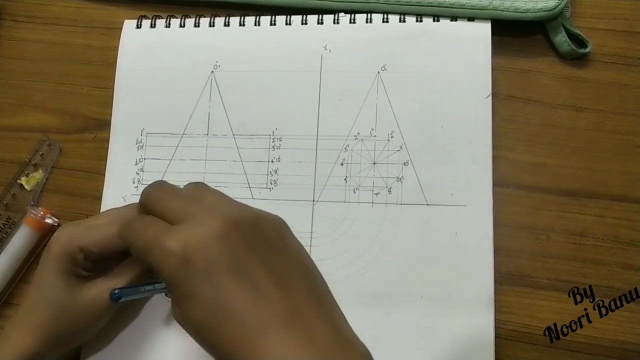 top view and combined side view. For getting the intersection curves here we have to take the first line, Okay, And take from this axis point to the second line, Okay, So this is 2. Send the middle point passing through this center by 2, or the middle point at the axis point passing through this center. 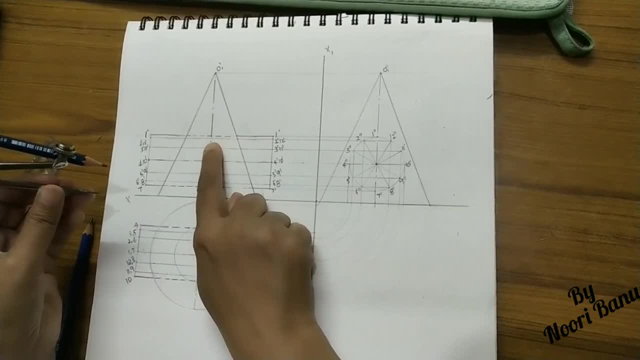 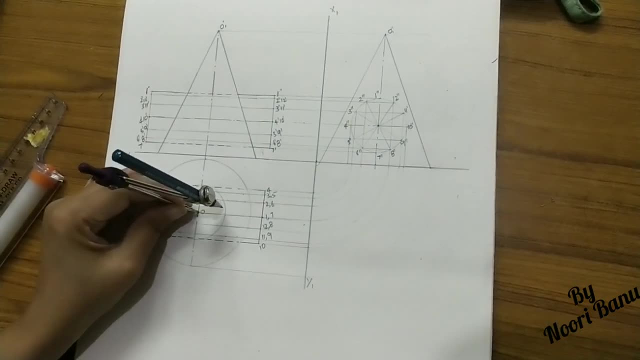 by 1.. Now on center block we have 3 round head, which 9 point. Okay. So once again this traveling over is we put on all the circle two times. So we have 7 artifacting side and we put round head. 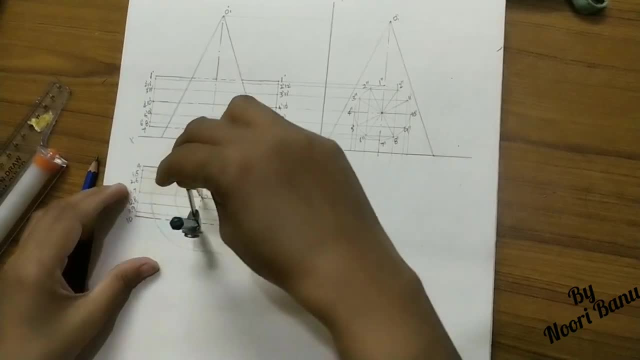 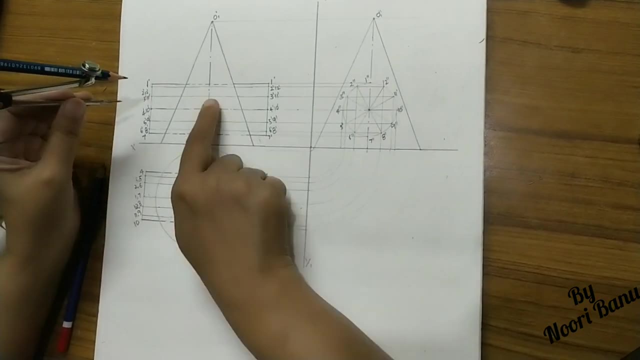 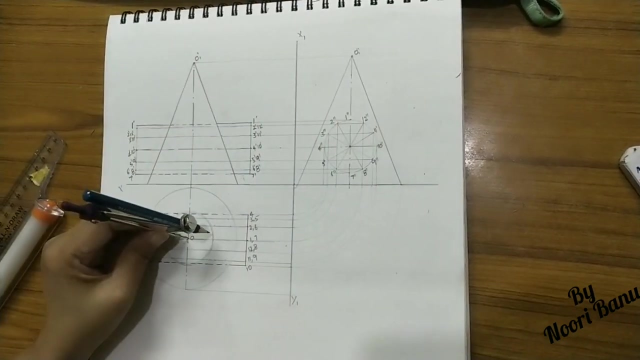 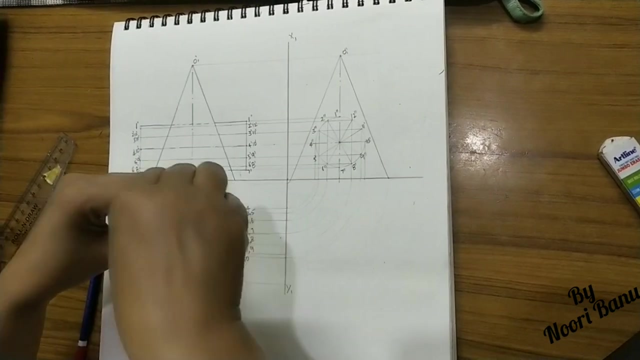 Okay, So this is our hill mark, If you look closely. Um now, after getting 2nd circle, take the 3rd line. take this distance as the radius. do one circle in the top, same point as center. do the 3rd circle. after that, take the 4th line. 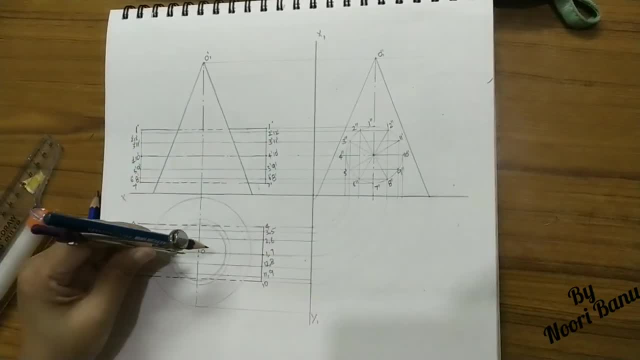 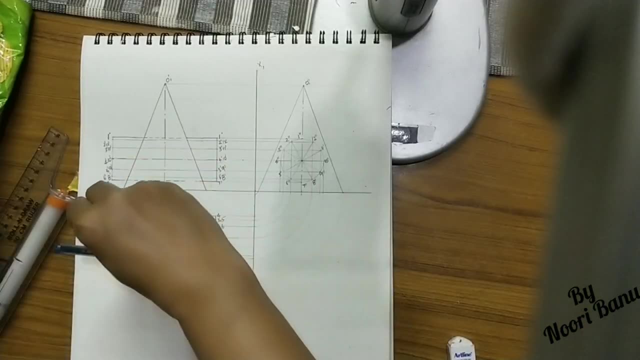 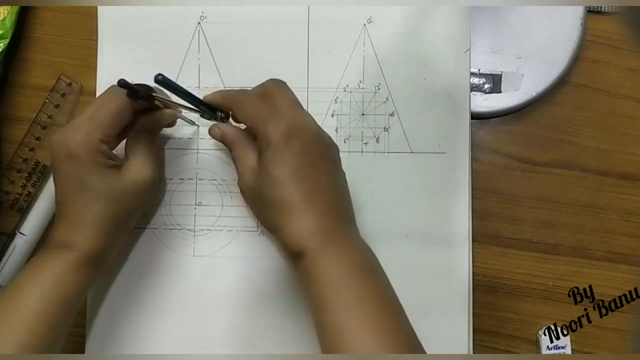 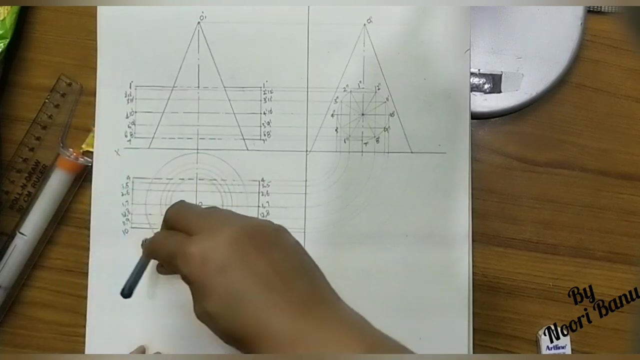 take this distance as radius, same center. do 4 circle. after getting the 4th circle, take the 5th, one, 5th line, from this point to this point as radius. so this is the radius, this point as center. do the 5th circle. 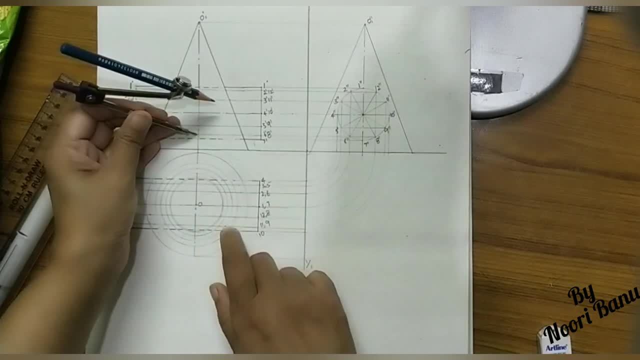 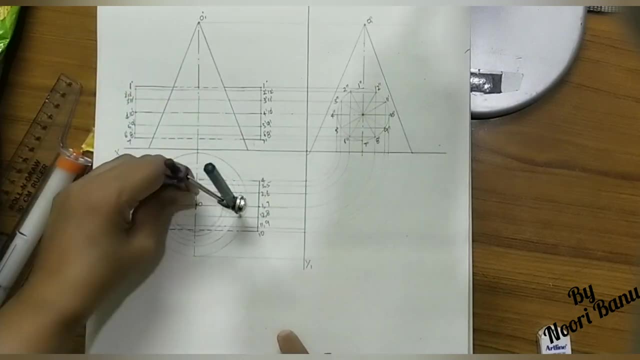 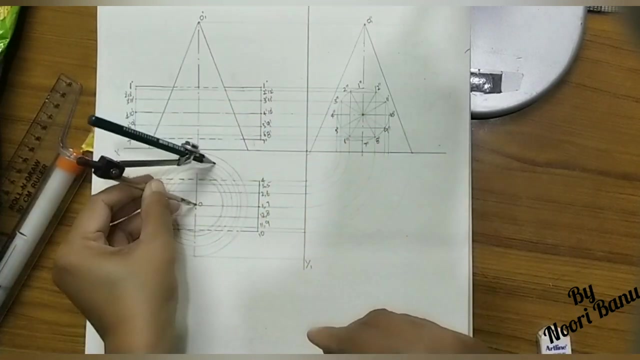 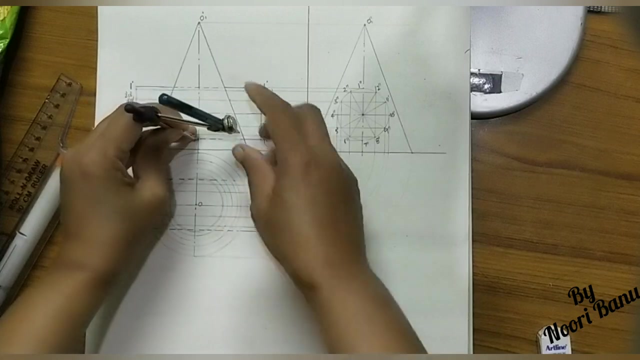 after getting the 5th circle, after getting the 3rd line, take this distance as radius circle. take the 6th line, this point as center. take this radius, this point as center. do 6th circle. after getting the 6th circle, take the 7th one, this point as center. and 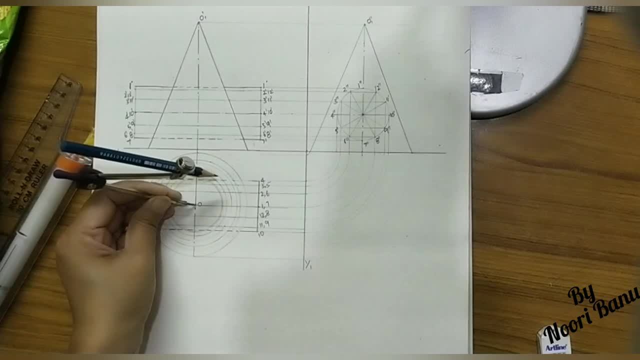 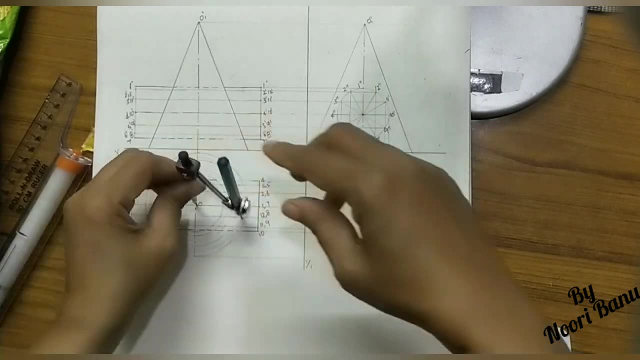 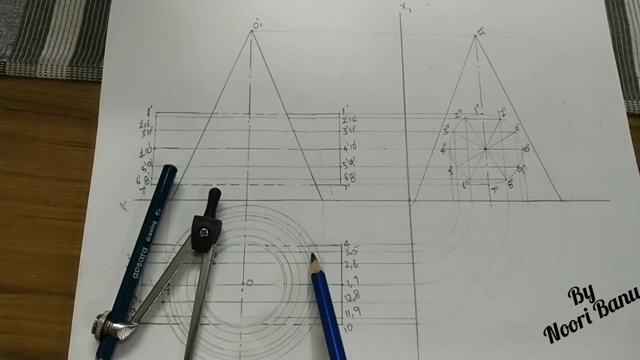 this is the radius. Do the 7th circle, this point as center. So by using compass here we did 1,, 2,, 3,, 4,, 5,, 6,, 7 circles. we did Don't take the outer circle. So up to here. 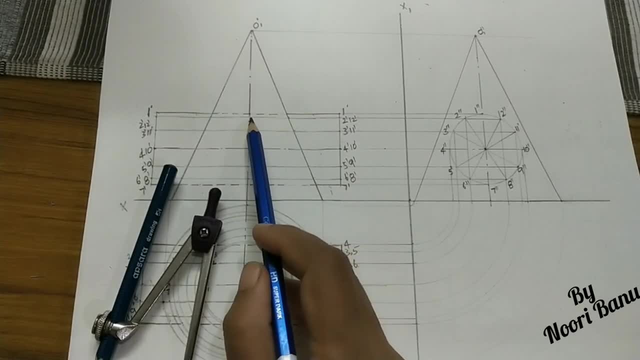 we did 7 circles Radius are. this is the first circle radius. this is the second circle radius. this is the third one. this is the fourth circle radius. 5th circle, 6th circle, 7th circle. 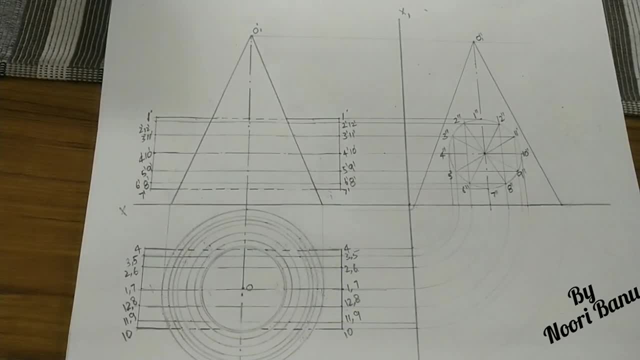 7th circle. Like that we did 7 circles. Now, after that mark the intersection points. Take the first circle and take the first line intersection point. So this is the intersection point, First line and the first circle. So I am marking this is P1.. This side I will 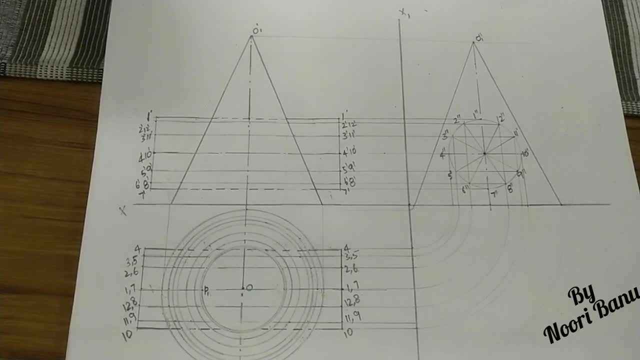 mark P1,, P2, P3, like that. This side I will mark Q1,, Q2, Q3, like that. And here, after P1, take the second circle, Take the second line, Take the intersection point. It is P2.. 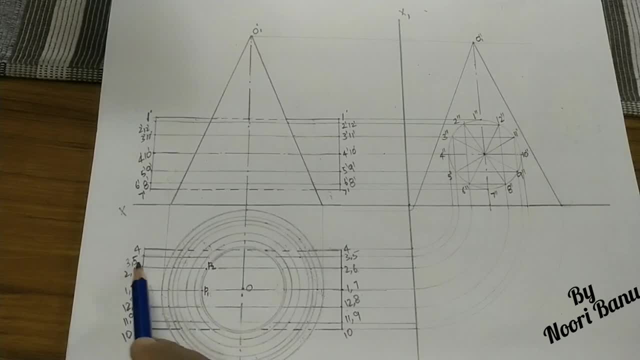 After P2, take the third circle and third line Take this intersection point is P3.. Next fourth circle and then fourth line Take this intersection point is P4.. Next take fifth circle and then fifth line. intersection point Take this point is P5.. So after fifth circle, take the. 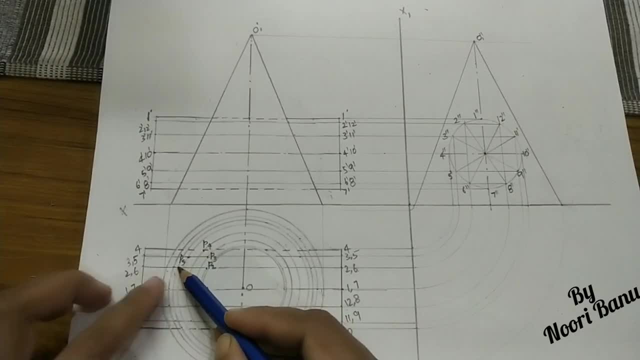 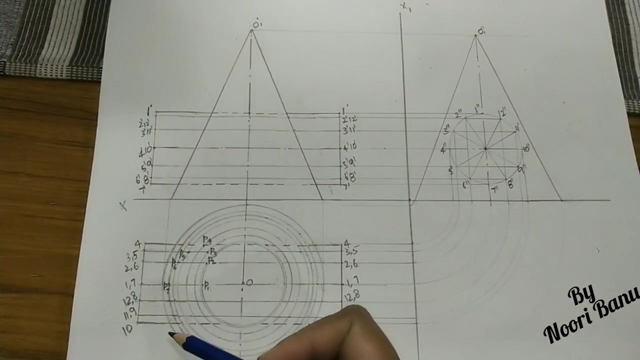 next circle. Sixth circle, Take the sixth line. The intersection point is P6.. Next seventh circle and then seventh line. The intersection point is P7.. Here, after marking P7, mark P8. Don't mark on the outer circle. Already I told, only take seven circles. 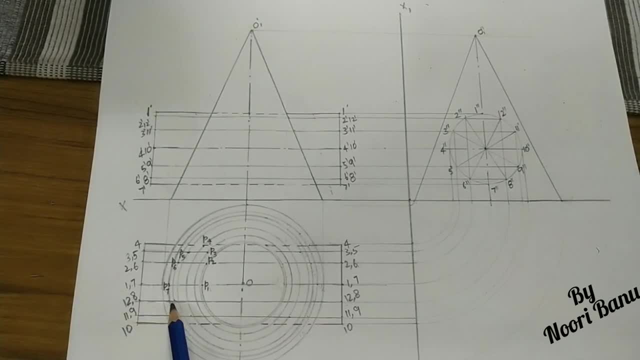 For P8, take the eighth line And then six and eight are coming on the same. Whatever sixth circle will be there, Take the same circle, Take the eighth line. So next circle After P7, next circle and eighth line. So this point is P8. So next P9. So already we did. 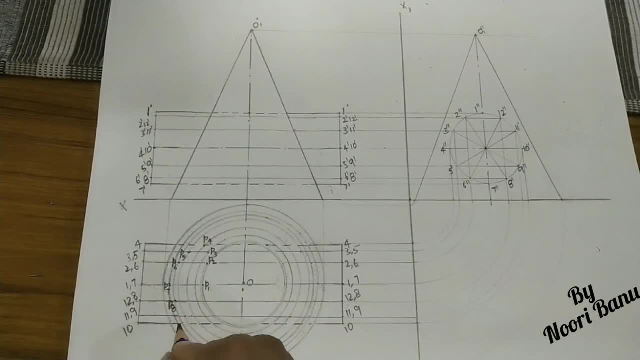 P8 here. Take the next circle. Take the ninth line, P9.. So after that P9, mark P8.. So after P10.. Okay, This circle we took. Now take this circle, Next circle. So mark this point is P10.. Next P11.. Take the next circle. Take the eleventh line, Mark P11.. Take the next. 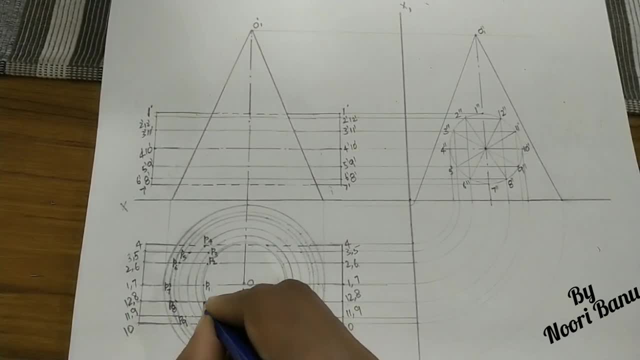 circle. Okay, Take the twelfth line, Mark here P12.. So we have marked from P1 to P12 points, All points. Similarly, this side also mark Q points. Take the first circle, First line, which is passing through one, Mark Q1 here. 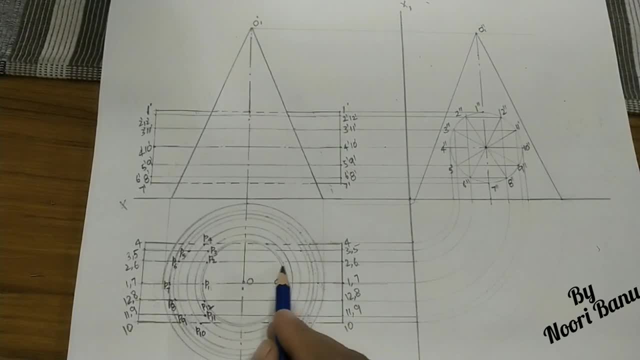 Next, second circle, Second line: Take the intersection point Q2.. Similarly, take third circle. Third horizontal line: Take the intersection point Q3.. Next, fourth circle, Fourth line Mark: this is Q4.. Just take one circle after another. Okay, After Q4, take the fifth one. 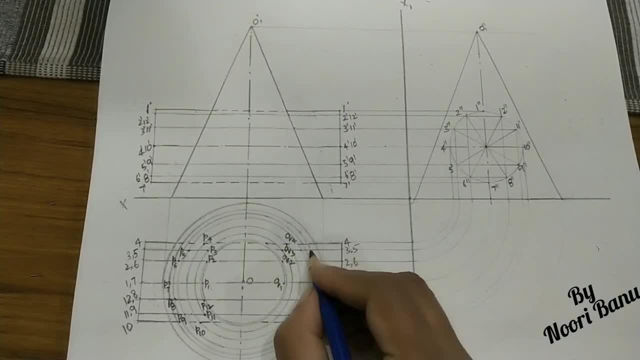 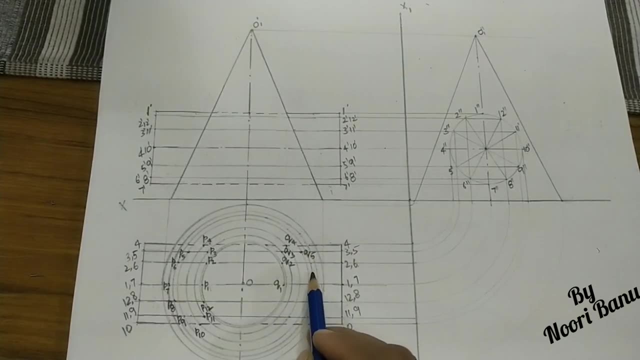 Fifth circle, Mark fifth point here. This is Q5.. This is Q5.. Next sixth circle: This one Sixth line Mark. this is Q6.. And then seventh circle, Seventh line, Mark: Q7.. Don't take outer one After Q7, mark Q8.. Okay, This on. 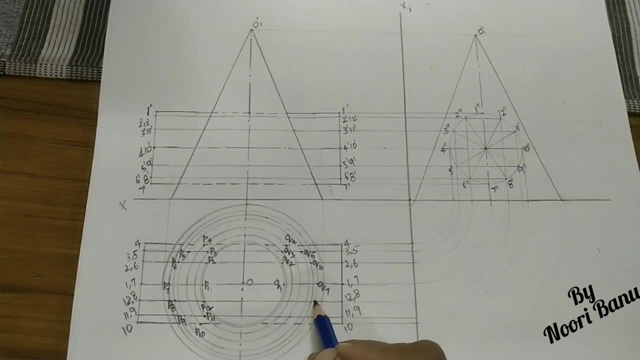 this circle we have marked Q7.. Q8 means next circle, And then eighth line, Q8.. And then next circle, Q9.. This is Q9. And then next circle, Q10.. And then next circle, Q11.. So this is eleventh line. 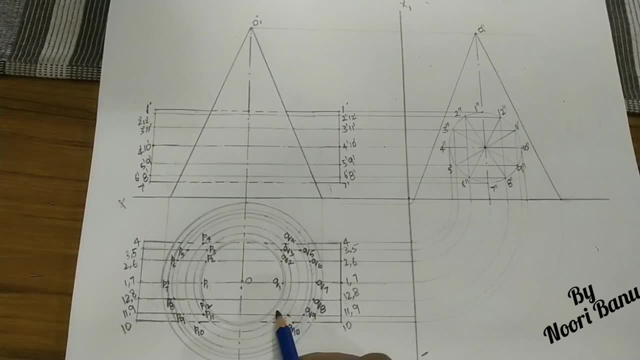 Next circle Q11.. And then next circle Q12.. Twelfth line: Like that from Q1 to Q12. we have marked all the points. So if you join all the P points, All the Q points, You will get the intersection curves in the top view. Try to join all the points. 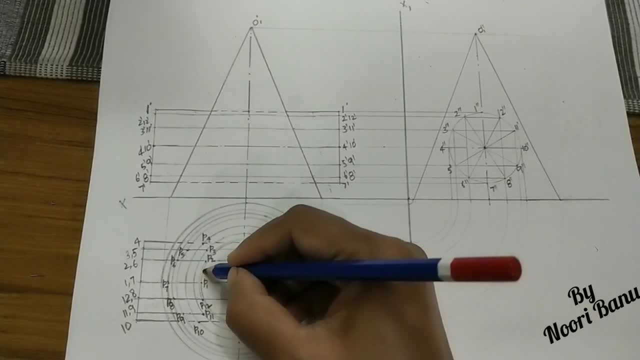 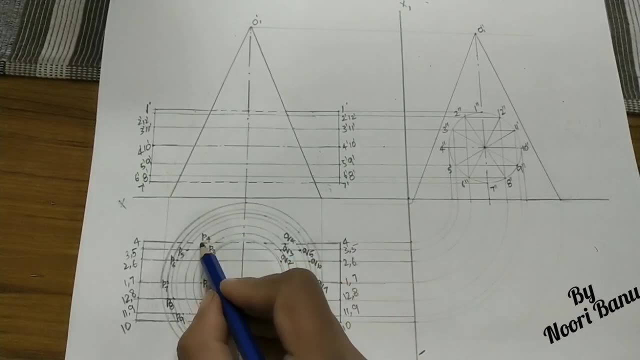 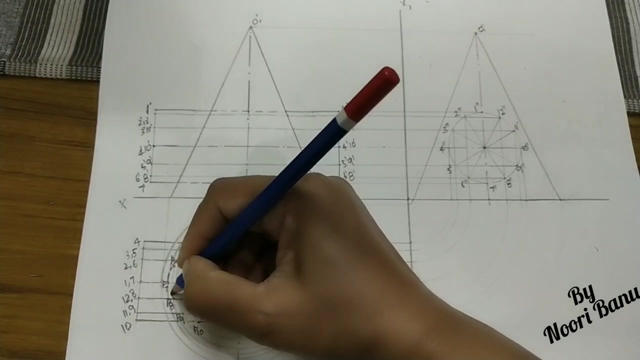 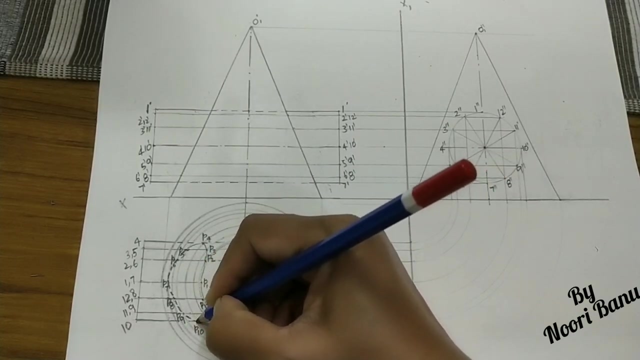 using freehand curve: P1 to P2, P2 to P3, P4, P4 to P5, 10.. So do this: outer points with dotted line. So P5 to P6,, P6 to P7, P7 to P8,, P8 to P9, P9 to P10 and then this inner: 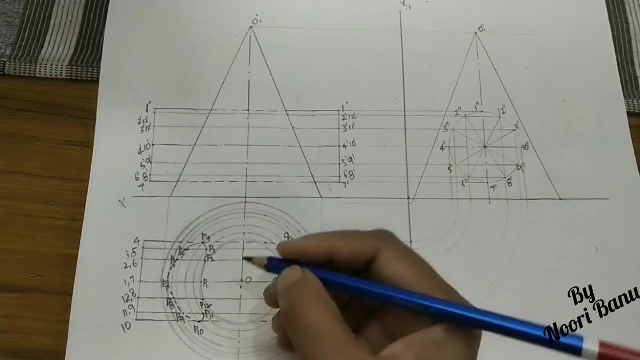 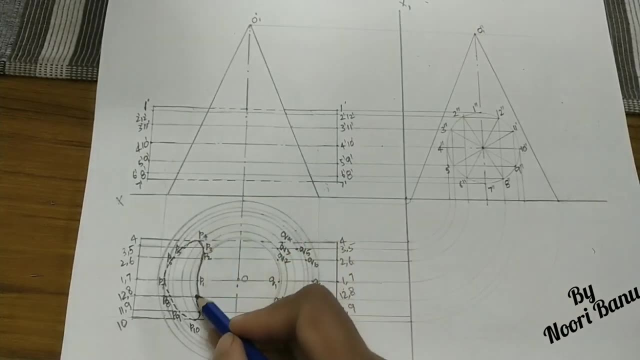 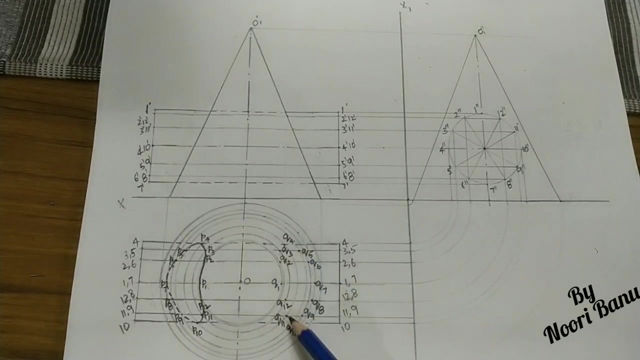 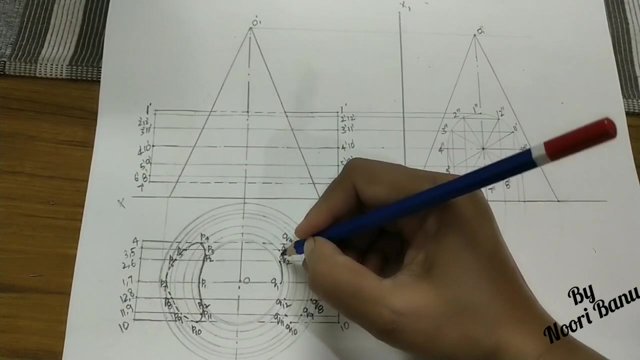 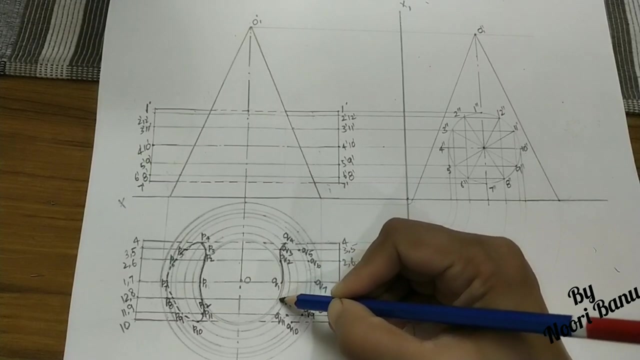 point should be with continuous curve, P11, P12 and then P1. So this curve should be, inner curve should be continuous And outer curve should be dotted. So here also inner point should be with continuous outer points with dotted Join: Q1 to Q2, Q2 to Q3. So similarly here also Q1 to Q12, inner. 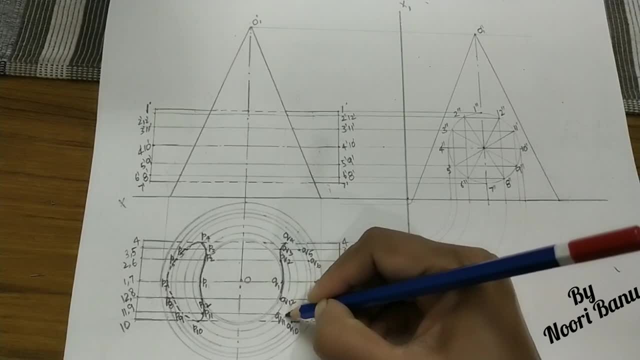 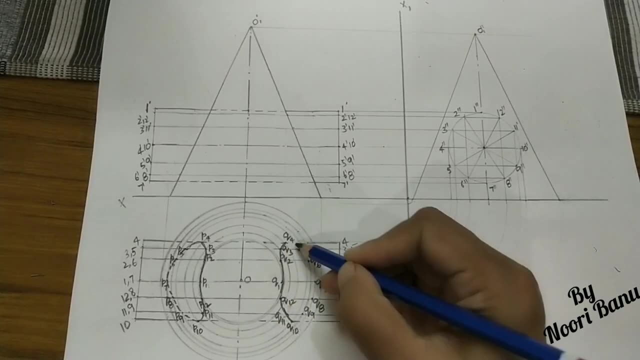 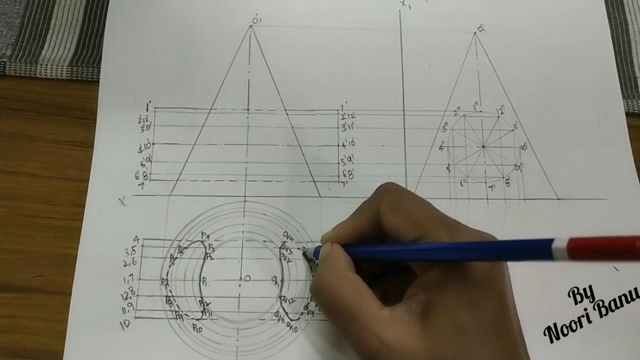 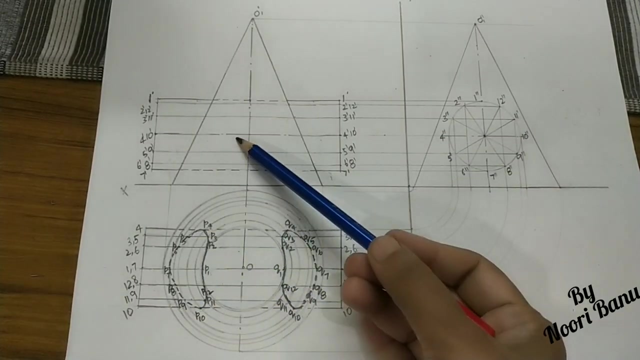 points. So Q12 to Q11 and then Q10.. So here these curves should be with continuous. So this curve should be dotted. These curves are the intersection curves in the top view. Mark these points, all these points in the front view, also P points as well as Q points. Now here take the P point. 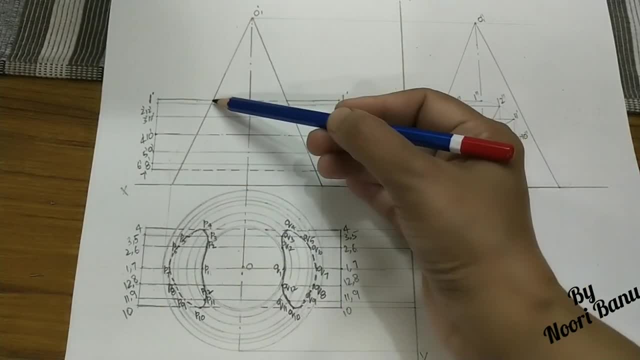 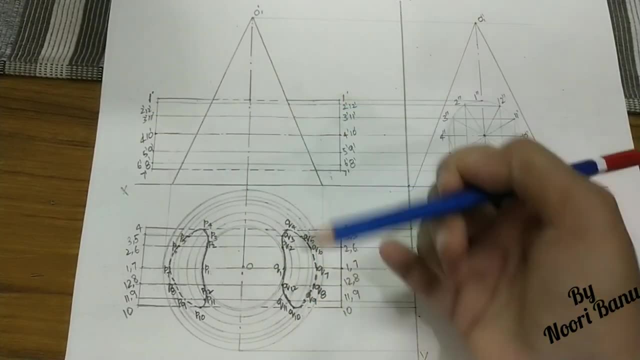 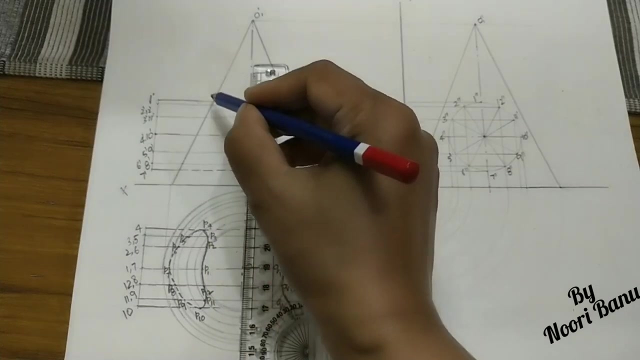 At P point. do the projector line up to first line Mark the top view point P1 dash. Similarly, take two point. Do the projector line Mark the intersection point. Like that you have to do the projector lines from all the points. Take this is the reference line From P1. do the line up to 1.. Take that intersection. 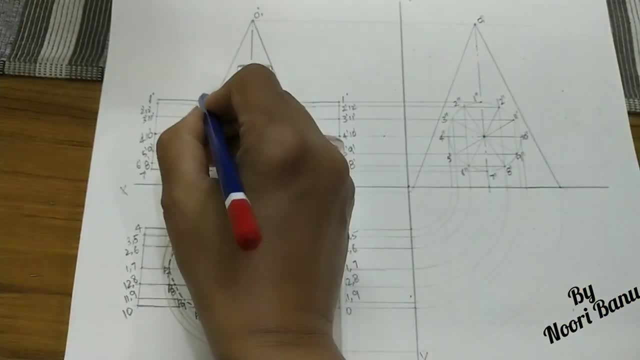 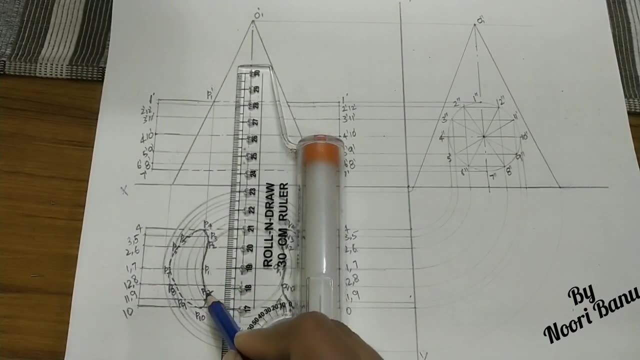 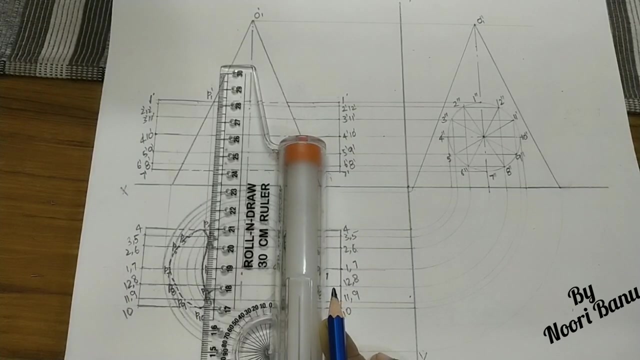 point. Okay, I am taking this is P1 dash. Similarly, take P2 and P12. Both are coming on the same circle. Okay, And if you do the line, these are coming on the same projector line: P2 and P12. Okay. 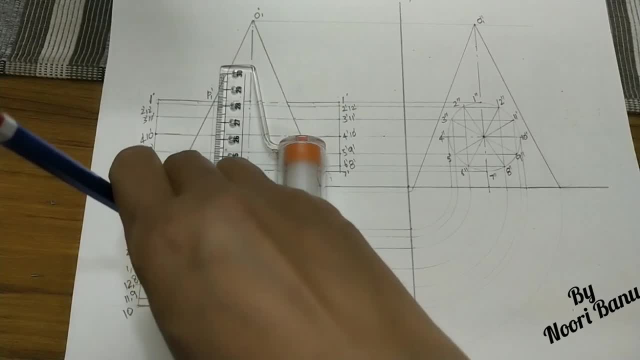 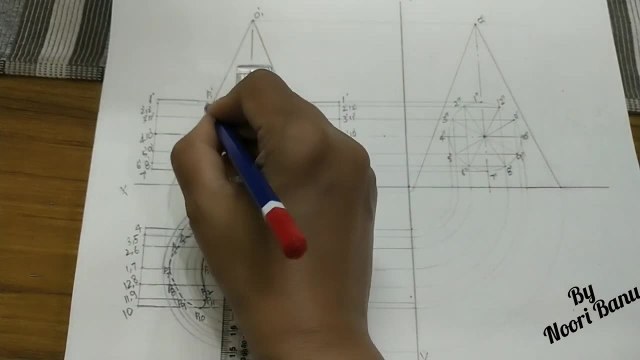 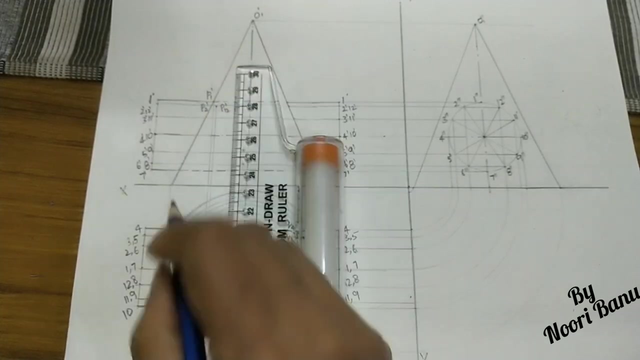 Here. this is P2.. This is P12.. If you do the line here up to 212 line, Okay, This intersection point is P2, dash Here one point. I will mark Here one point. I will mark P12, dash Okay. 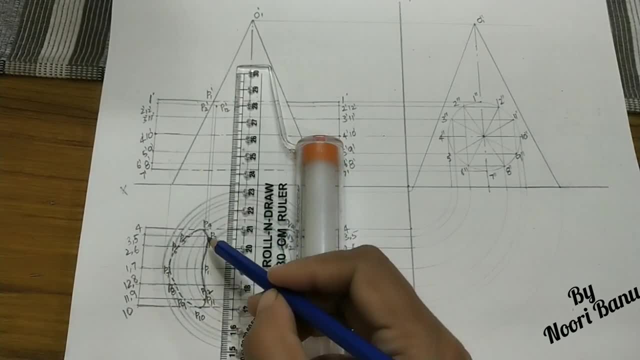 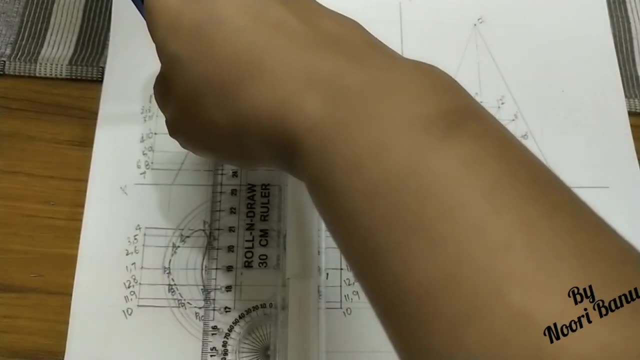 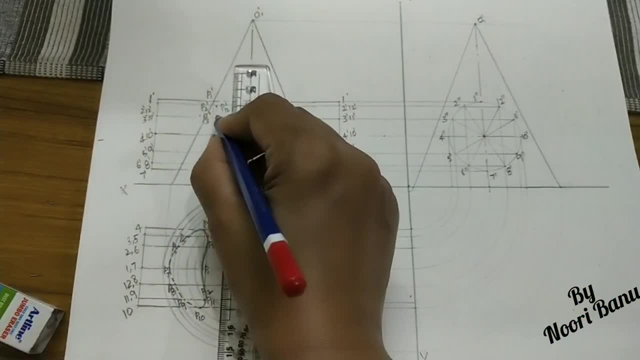 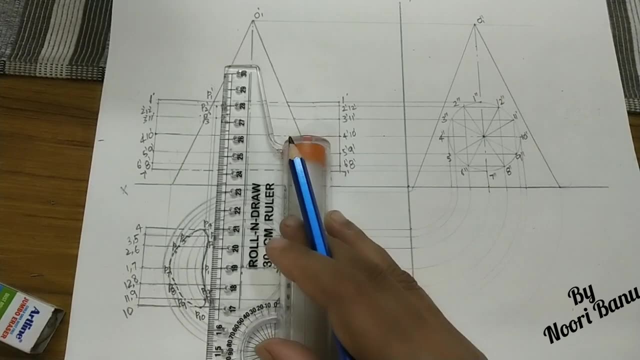 Okay, Okay, Okay, Okay, Okay. P3 dash, P11 dash. After that, after 3 and 11, take 4 and 10.. Okay, If you do the line, both are coming on the same line, Okay. 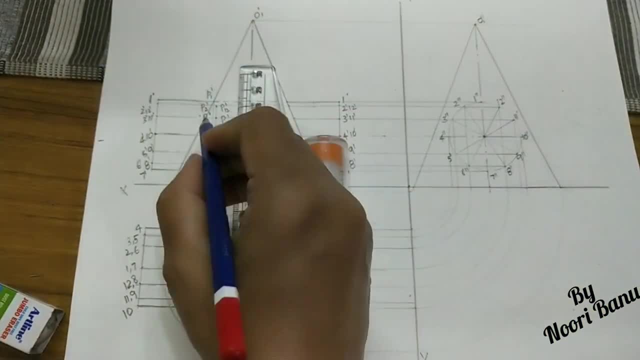 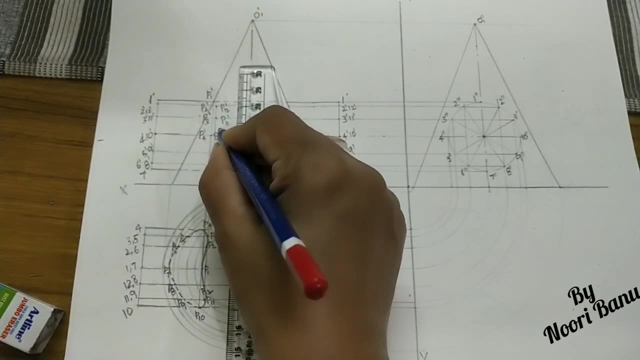 Do the line here: 4 and 10.. So this point is P4 dash and this side I will mark P10 dash. Okay, These points. okay. 4 and 10. I am marking at this point, After 4 and 10, mark 5 and 9.. 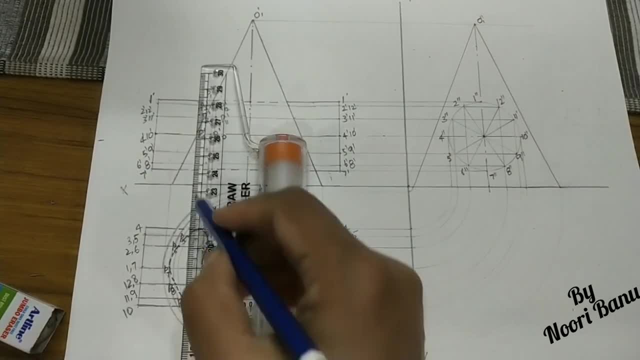 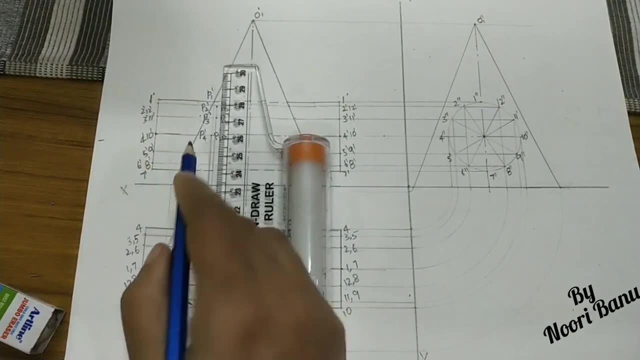 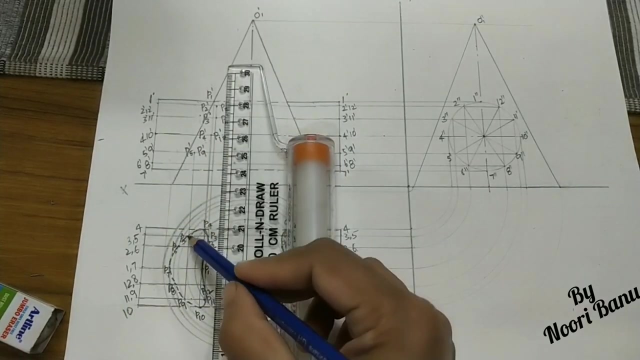 If you do the line here, 5 and 9 are coming on the same line. Do the projector line here up to 5 and 9.. Okay, So mark this side: P5 dash, P9 dash. After 5 and 9, take 6 and 8.. 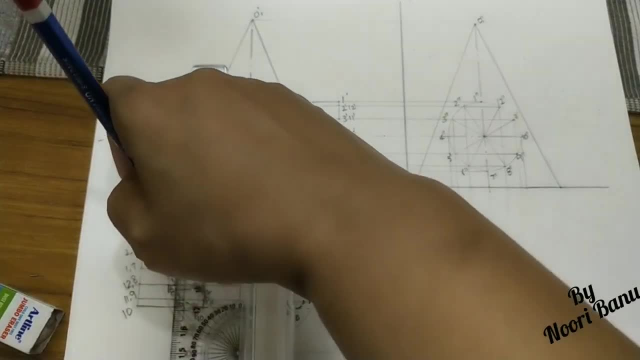 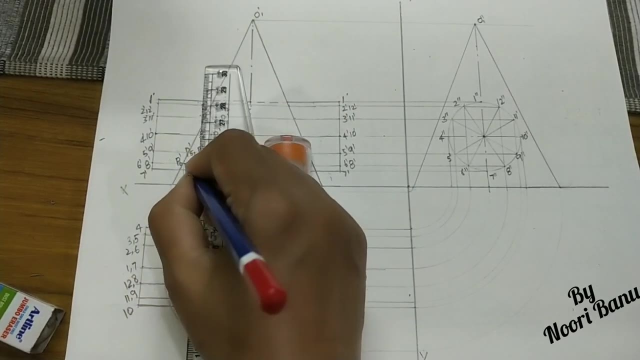 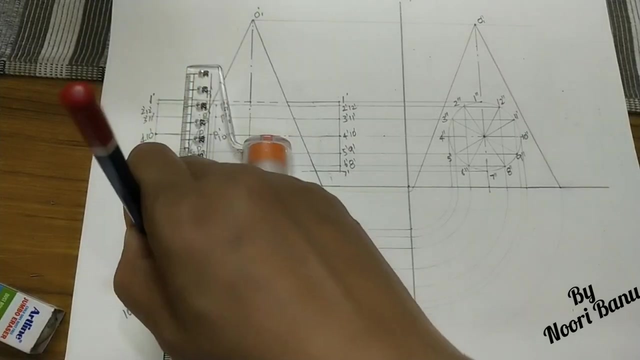 Both are coming on the same line. Okay, Do the projector line here up to 6 and 8.. Okay, This point, So up to 6 and 8, P6 dash, P8, dash. After that last point is P7. 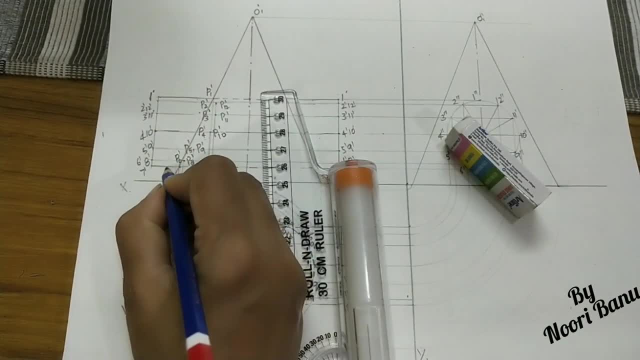 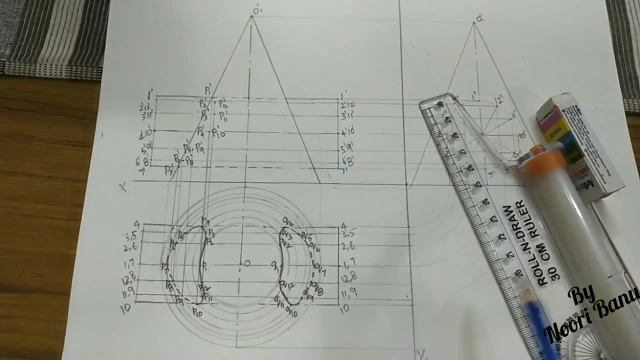 So do the projector line here. So it is a starting point here. So it is P7 dash. Okay, It is the last point. This is the starting point Now. similarly, mark Q points also here. Okay, This is the reference line. 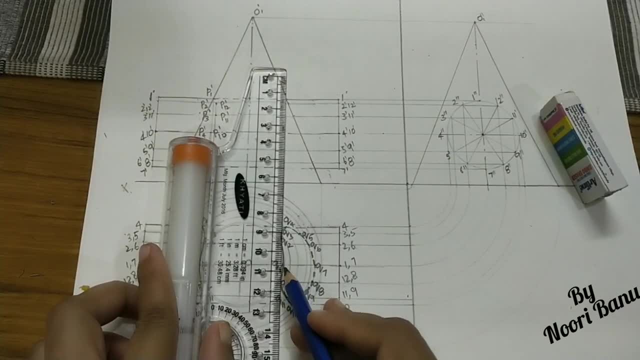 Move up to Q1.. Do the projector line up to 1st line? Okay, From Q1 to 1.. This is Q1. dash Getting 1st point. Take 2nd one, 2nd and 12.. 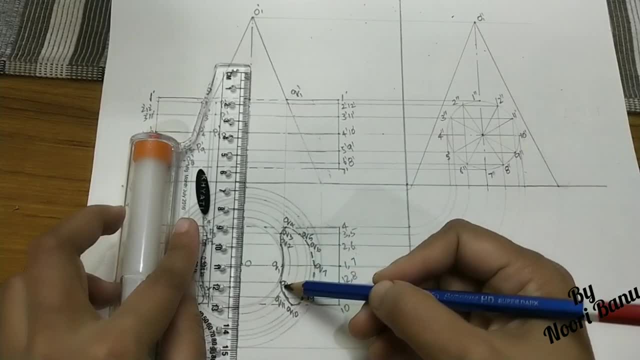 Both are coming on the same circle. Move the scale up to Q2 and Q12.. Here Q2,, here Q12.. Just do the line here. Okay, This point is Q2, dash, Q12, dash. Okay, Up to 2,, 12.. 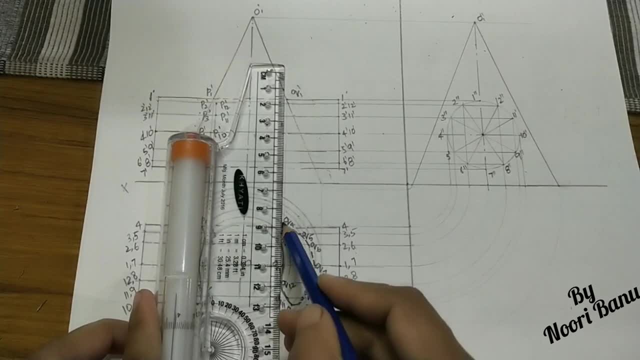 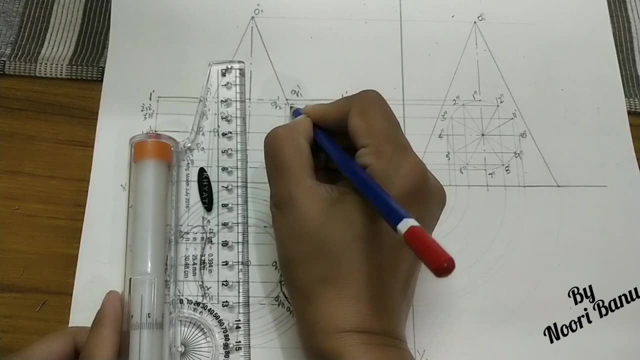 Okay, After Q2, take Q3.. Q3 and Q left. Okay, This is Q3.. This is Q3.. This is Q4.. This is Q5.. This is Q6.. This is Q7.. This is Q8.. 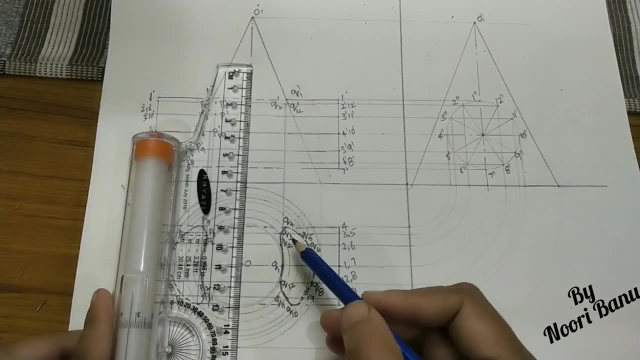 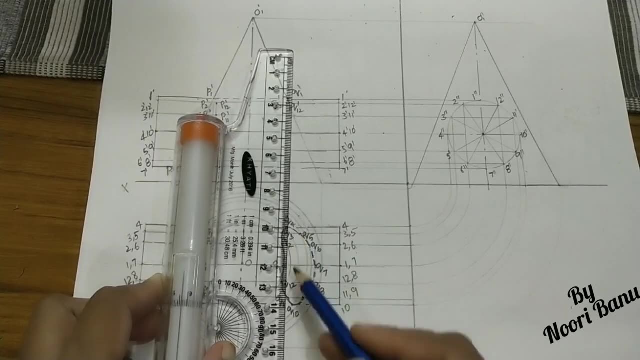 This is Q9.. This is Q10.. This is Q11.. This is Q12.. This is Q12.. This is Q3.. Q3 and Q11 are coming on the same line. Move the scale. Okay. Q3, Q11.. 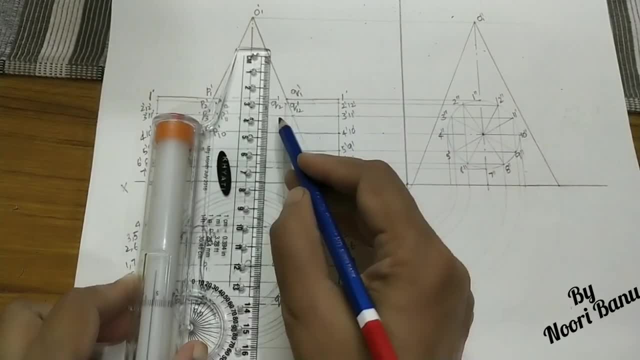 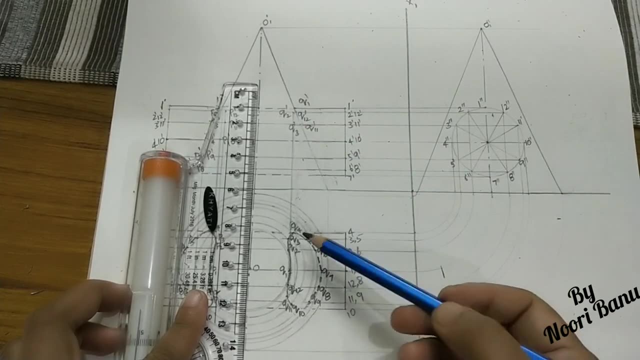 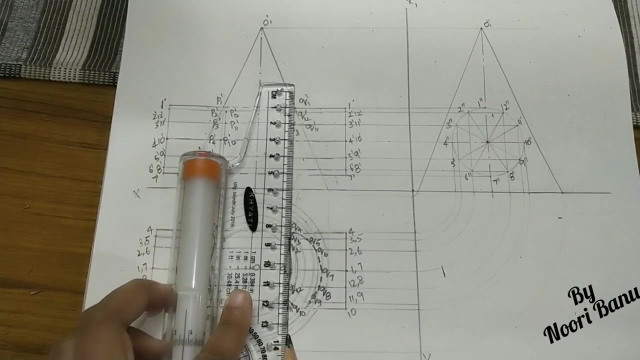 Do the line up to this: 3, 11.. Okay Here, Q3 dash, Q11 dash. After Q3, point mark Q4.. Q4 and Q10: both are coming on the same circle and same line. Move the scale up to Q4.. 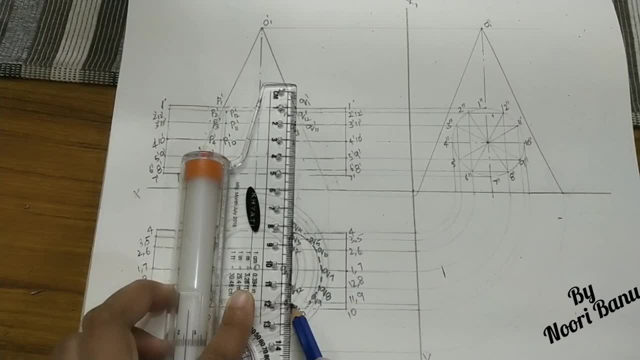 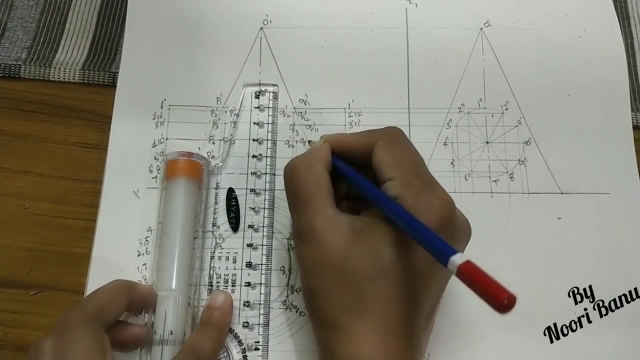 So this is Q4 point. This is Q10 point. Do the line here up to 4 and 10.. Okay, Mark, this point is Q4 dash and Q10 dash. So after marking Q4, mark Q5.. 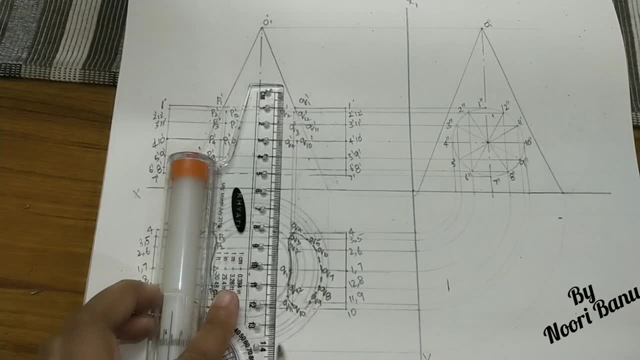 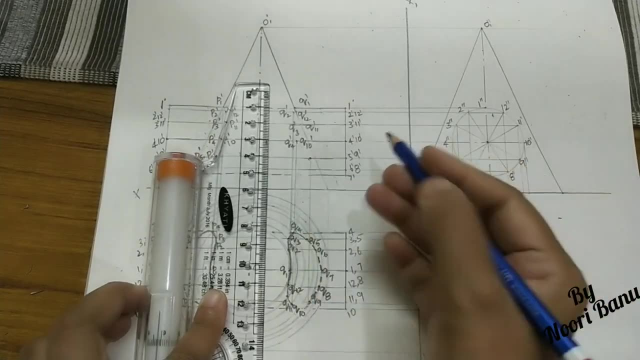 Okay, Q5 and Q9. both are coming on the same line. Move the scale up to Q5.. Do the line up to 5, 9.. Okay, Mark, here point Q5, dash, Q9, dash. After Q5, mark Q6. 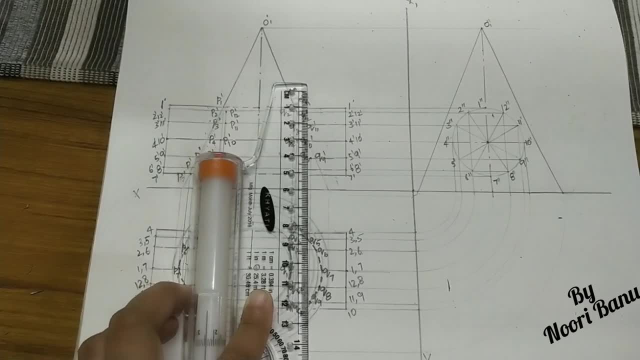 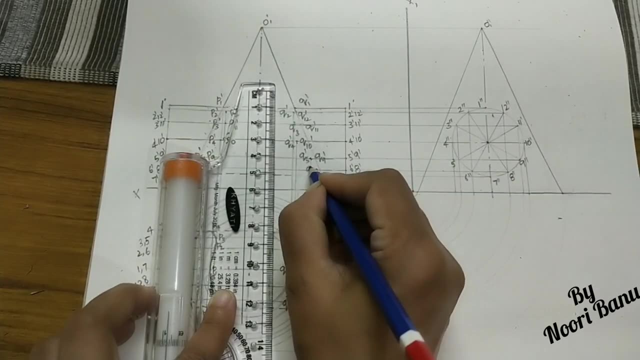 So Q6 and Q8. both are coming on the same line. Move the scale up to here: Q6 and this is Q8.. Do the line here up to 6 and 8.. So mark Q6 dash, Q8 dash. 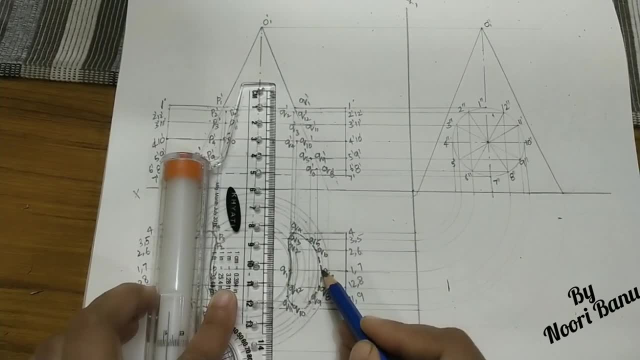 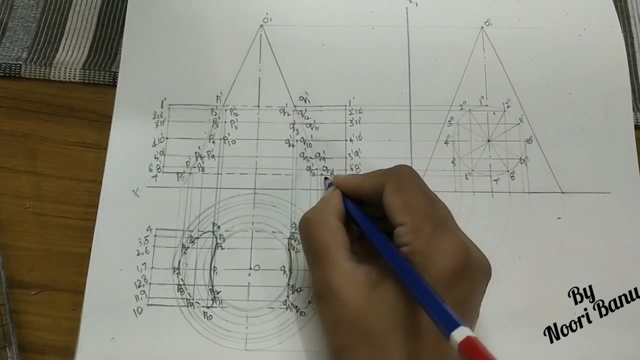 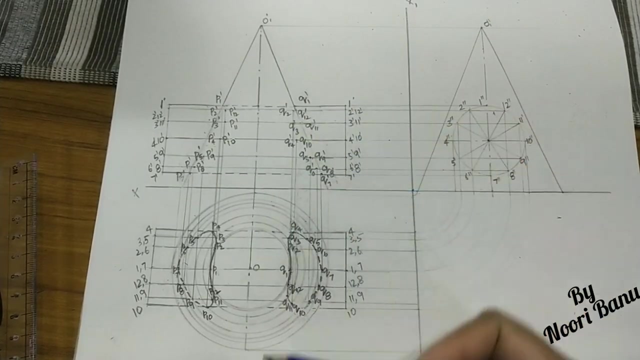 After that last point, After Q6, mark last point Q7.. Do the line projector line here up to this. So this is the last point, Q7. dash, If you join all these points from P1 to P7 and Q1 to Q7, we will get the intersection curves in the front view. 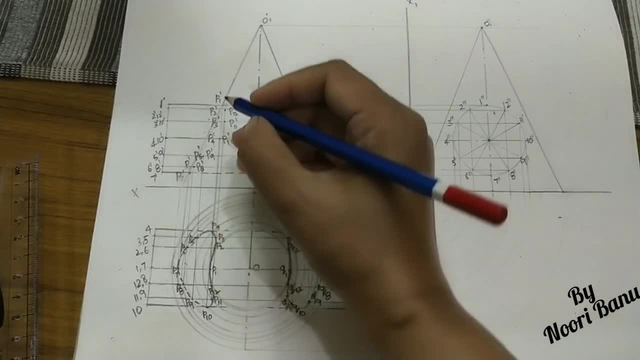 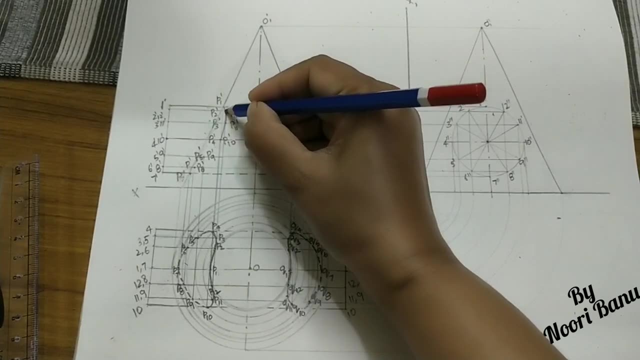 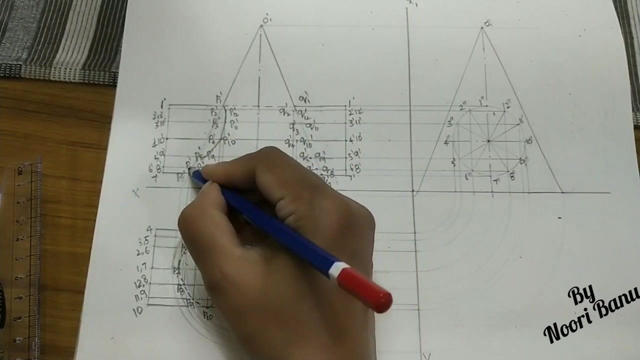 Okay, Let us do the curves by using free hand. curve P1 to P2, P2 to P3, P3 to P4, P4 to P5, P5 to P6,. this is P6.. P6 to P7. 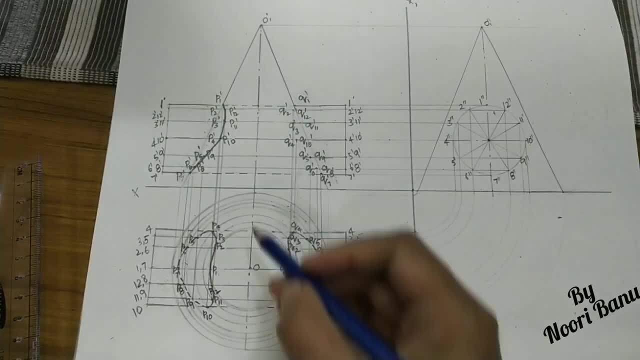 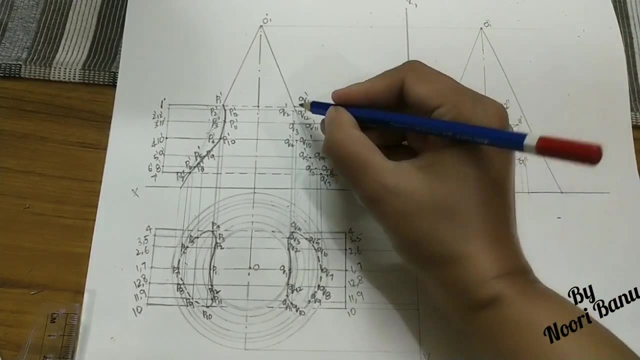 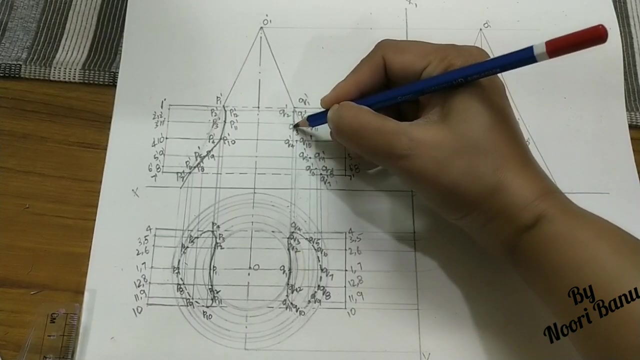 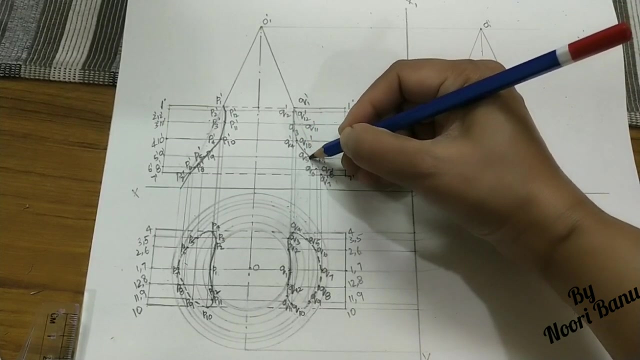 Okay, This is the intersection curve in the front view. Similarly, join these points also from Q1 to Q7.. By using free hand curve: Q1 to Q2, Q2 to Q3, Q3 to Q4, Q4 to Q5, Q5 to Q6, Q6 to Q7. 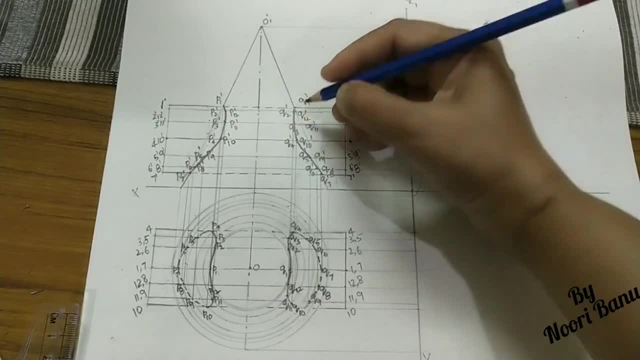 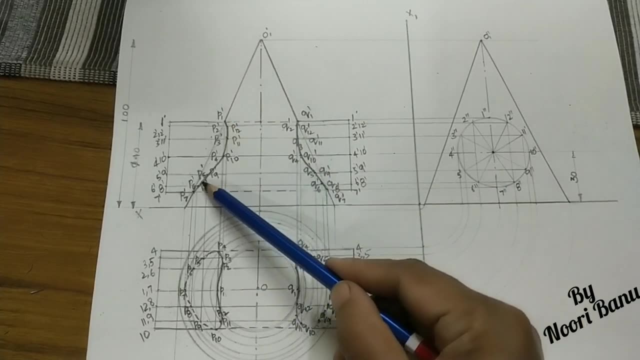 Make it dark. And now these are the projections of the combination of two solids. This is the front view, This is the top view, This is the side view And these are the intersection curves. And in the top view, these are the intersection curves. 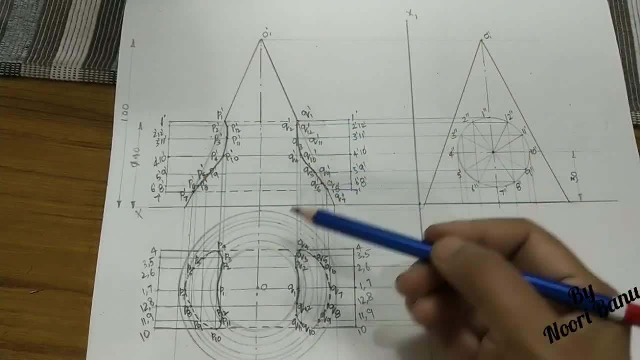 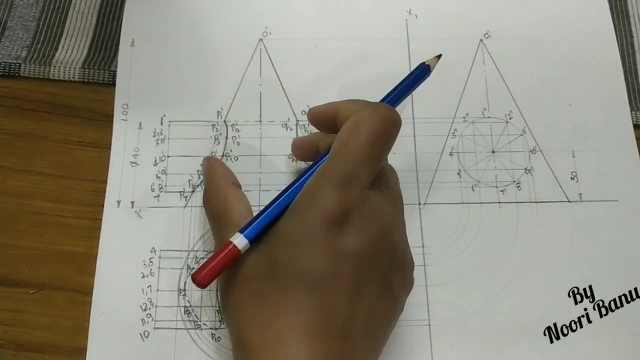 Okay, And here, make this curve should be in dark color. And this is the cone. Okay, This is the cylinder. This line should be in light color Because this cone we are inserting into this cylinder. Okay, And the intersection points.